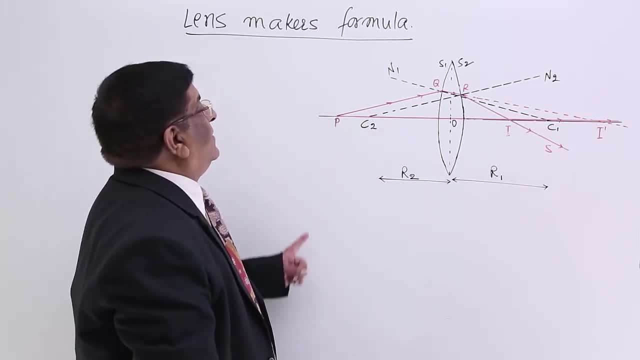 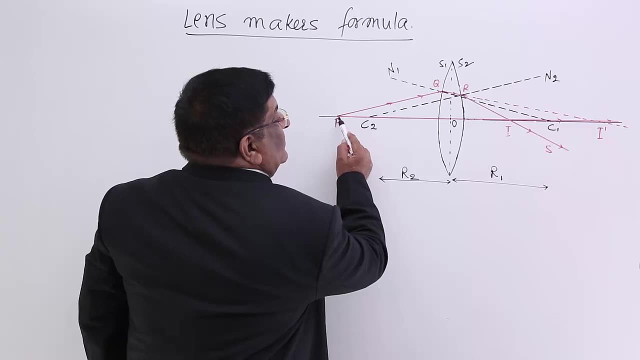 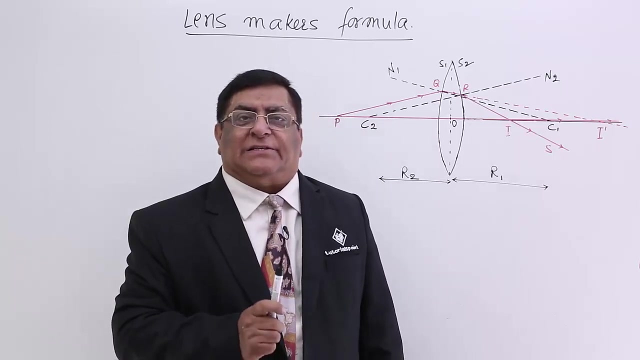 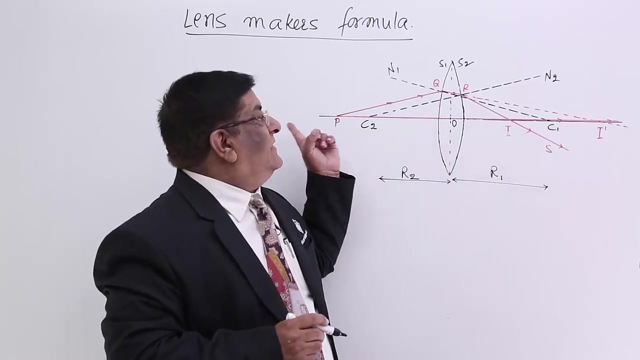 call it r2.. Now we have taken one object at this point P From this P, it will be this point R2.. 1 ray, which is along the principal axis. How do we decide the principal axis in this case? In this case, when we join the 2 centers of the 2 surfaces, center 1 and center 2, this 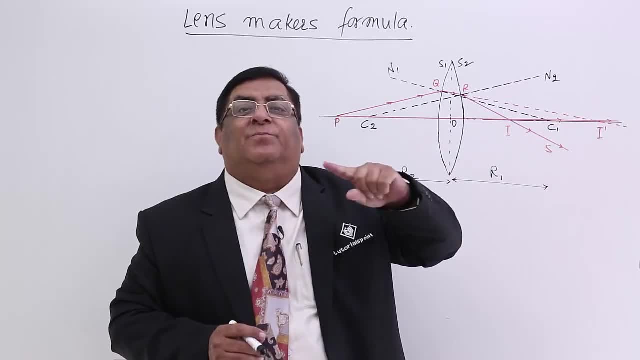 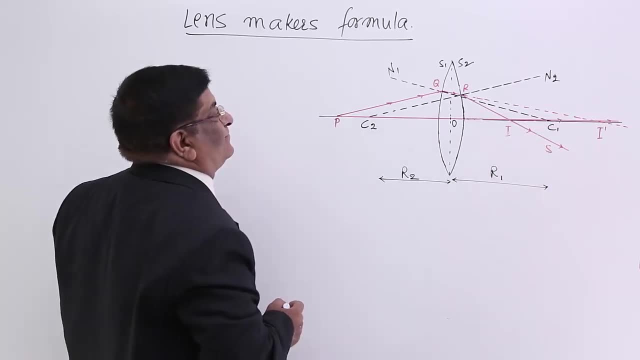 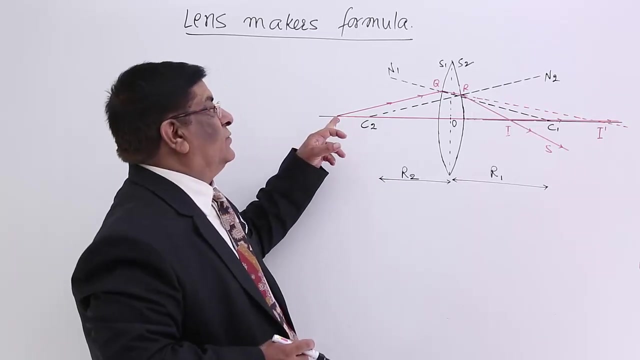 line extended on both sides will be known as principal axis of the lens. So this is principal axis of the lens. There is one point P on the lens where we are placing the object. This is the source of light. 1 ray is going along the principal axis and we are trying. 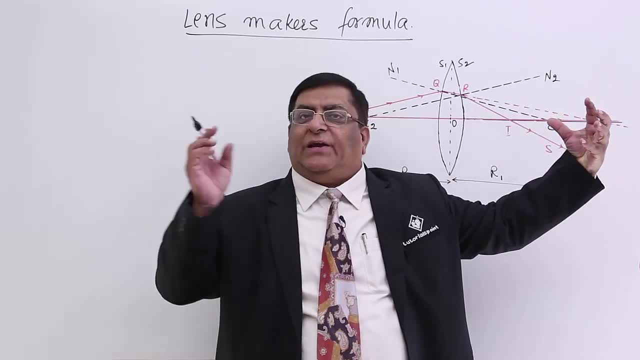 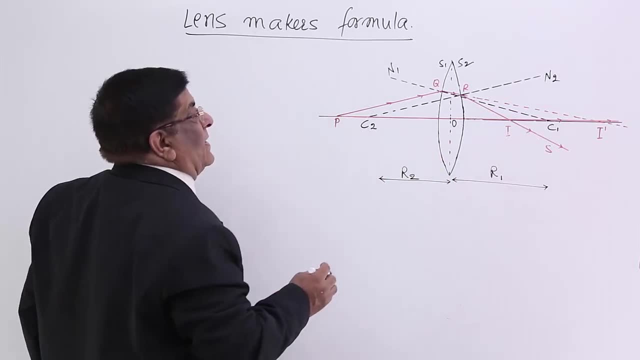 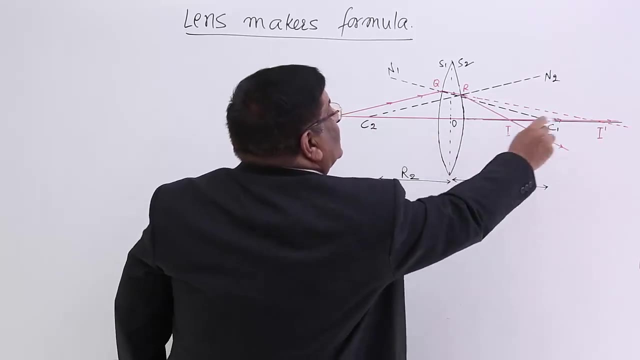 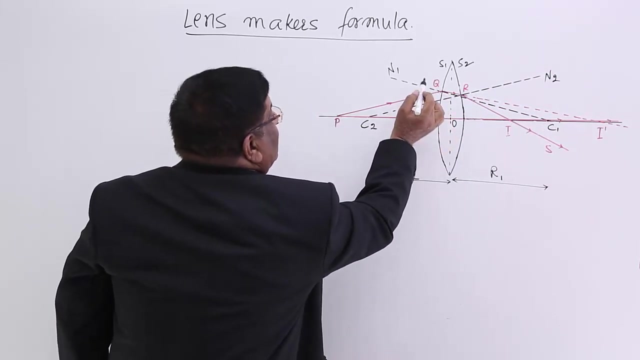 to see it from this side. Here is the object where we keep the lens, Here we keep our eyes to see the object Now, 1, This is the source. From here we take 1 ray along the principal axis which goes straight along the principal axis. The 2nd ray we take which is going anywhere towards the lens. 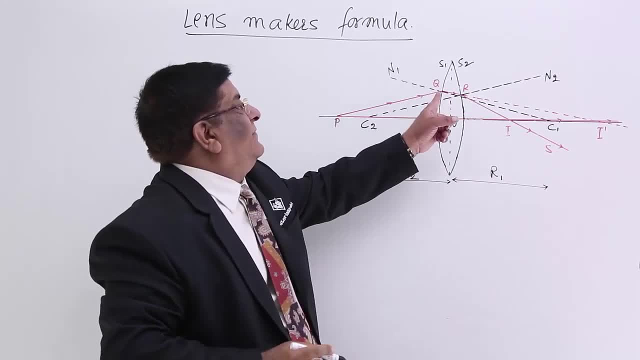 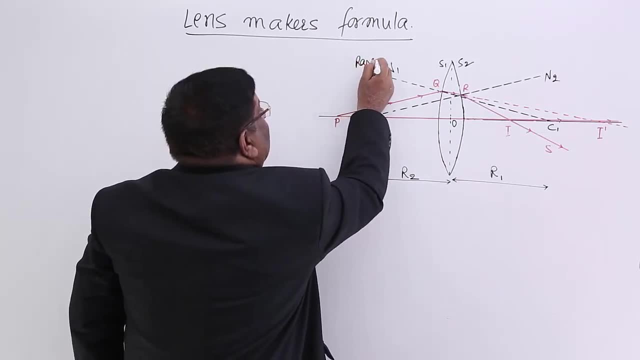 Let us see: it strikes the 1st insert face, 1st surface at point Q, Then what will happen? It is going from rarer medium, This is rarer, and this is denser medium. Then again, this is rarer medium. 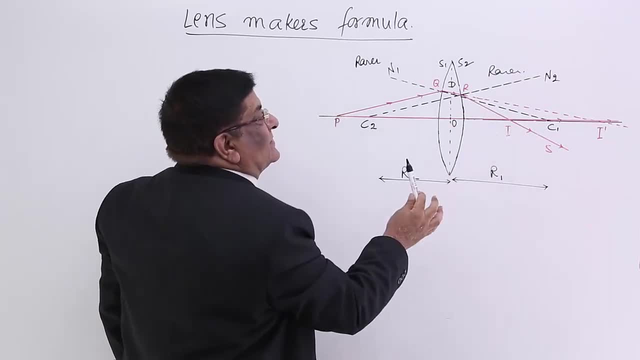 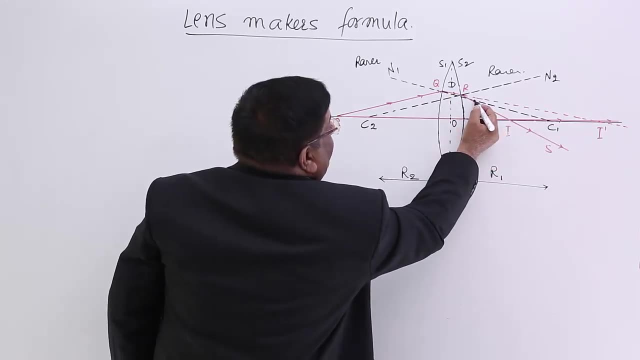 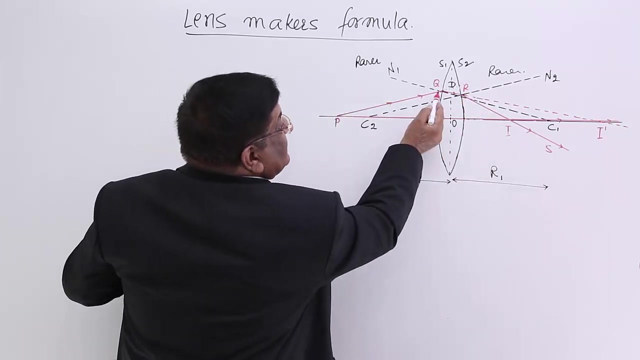 It is going from rarer to denser, so it will bend towards normal On the surface. 1 when we connect it with c1, this line represents the normal. Now, this ray which was going straight, otherwise this way it was going, but it has to bend towards normal. This is the normal. 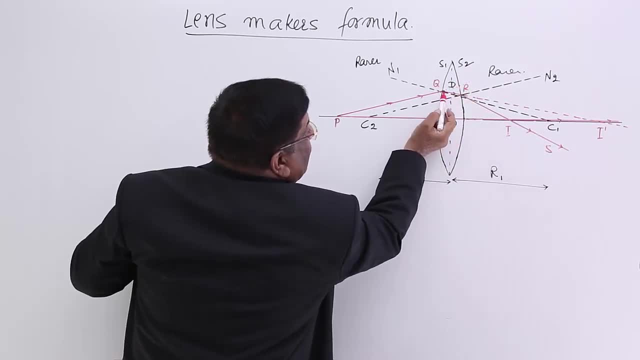 so it bends towards normal this way And this is how it is going. This is the normal. This is the normal. Then again, this is rarer medium, this is denser. Then again, this is going from rarer medium to denser. Then it will bend towards normal. And when we connect with the point, 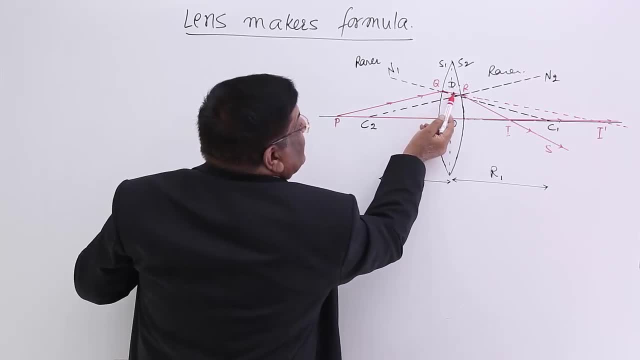 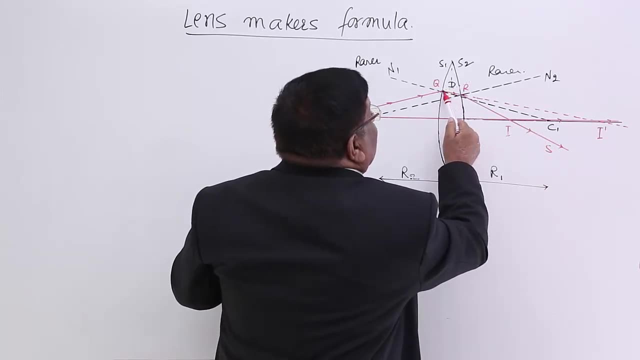 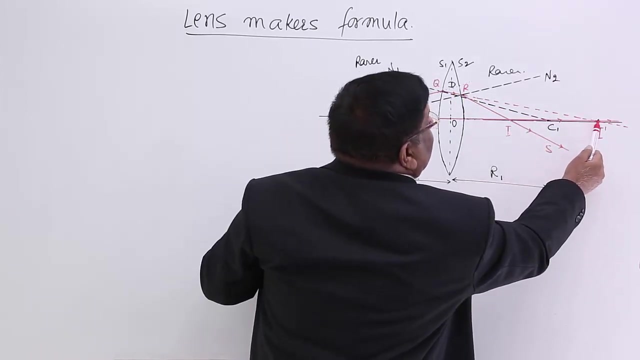 it travels. Now, when it is travelling this way it has. if it keeps on travelling in this medium, denser medium, then it is supposed to strike at this place with this second ray and this will make a image here. So the first surface decided that I will bend the light. 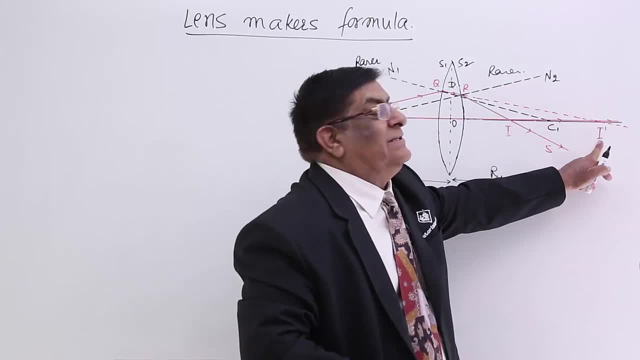 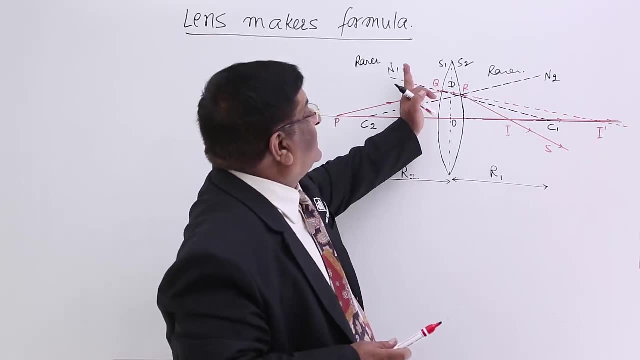 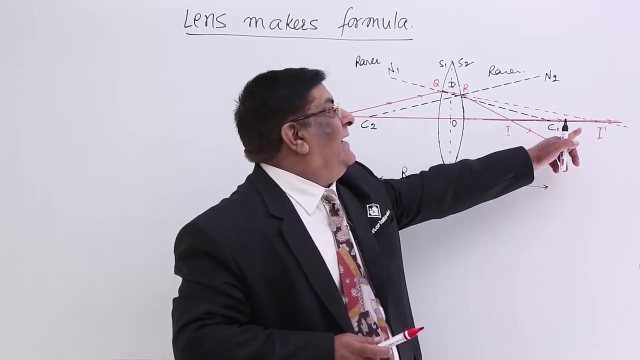 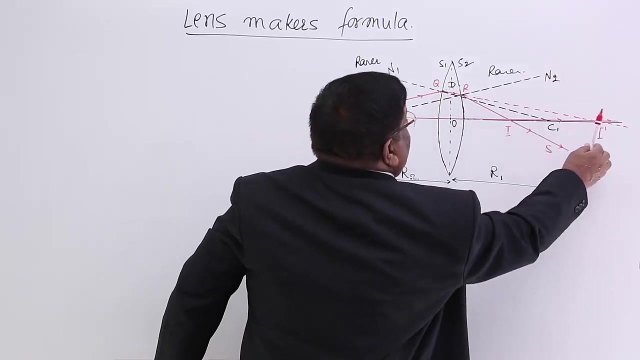 in such a way that it will make a image at this point, and this is the name we have given: I dash. So, due to first surface of this denser medium, the image was being formed at I dash but could not be formed. Why could not be formed? Because this medium is not all the 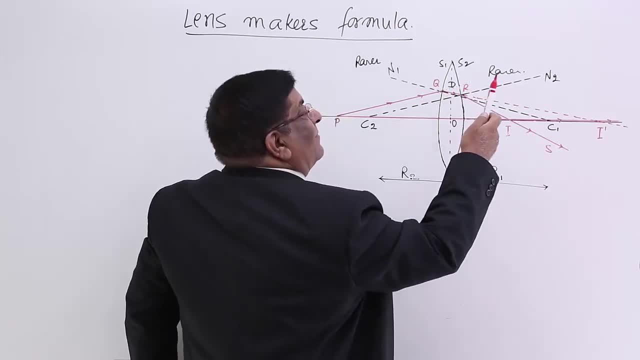 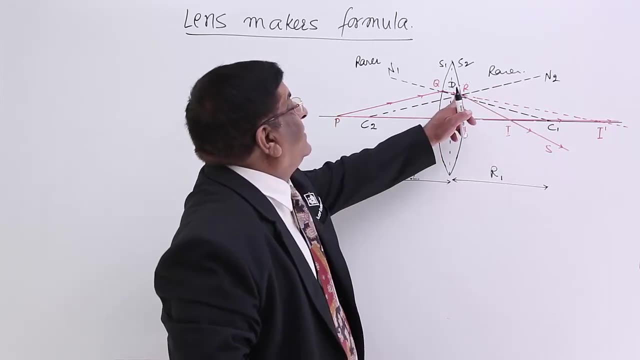 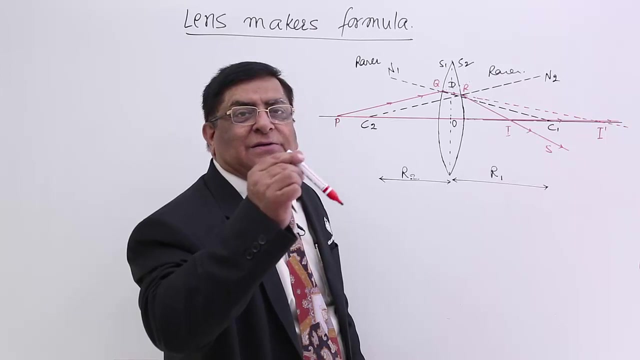 through. By the time this ray reaches here, the medium has again changed And now it has become rarer again. So it could not travel further. because the ray travel in one medium straight. When the medium change, it will bend. Now the medium has changed from. 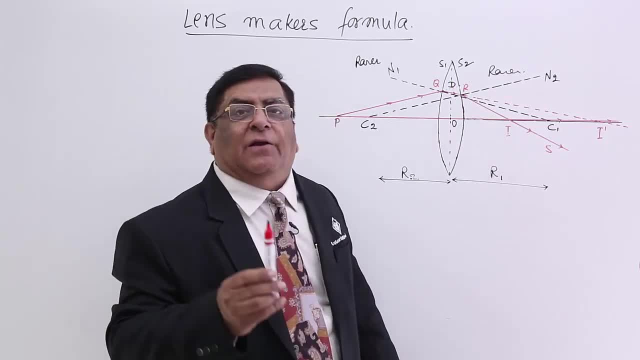 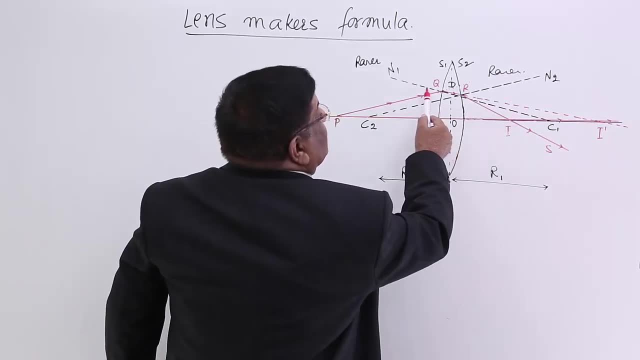 denser to rarer. and what is the rule? It will move away from the normal. Where is the normal Now? this normal will not do because this was the normal on the surface one. This is the reflection at surface two. So we draw a normal of the surface two. This is normal on the 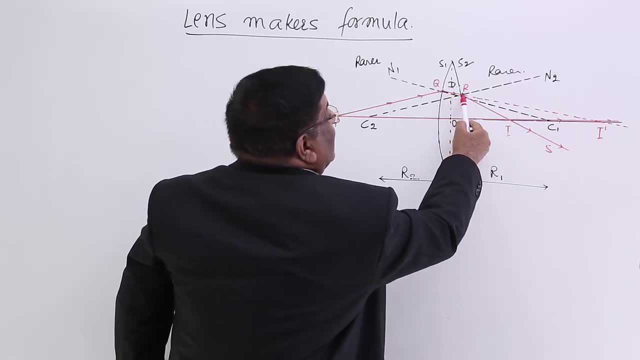 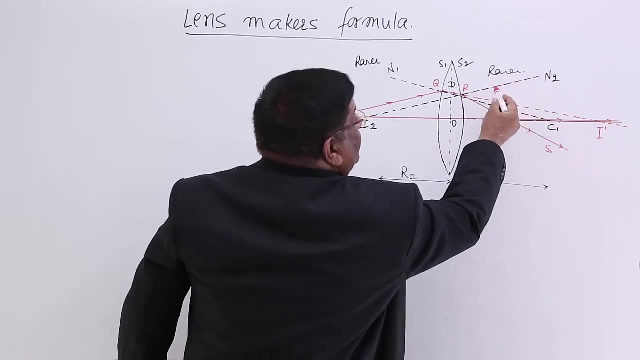 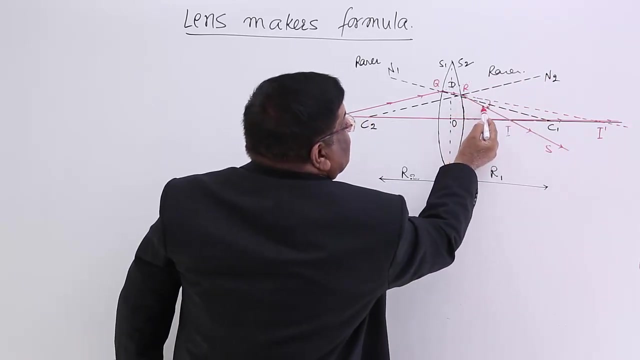 surface two, and what will be it? fate Answer is this: one was going in this direction. now it should move away from the normal. This is the normal for surface two and it will move away. So it moves away this way and this is the new path in this rarer medium With 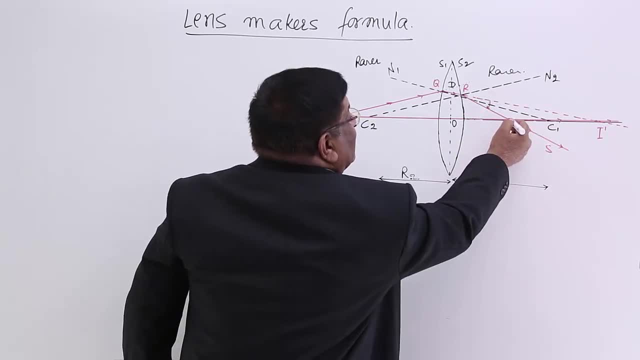 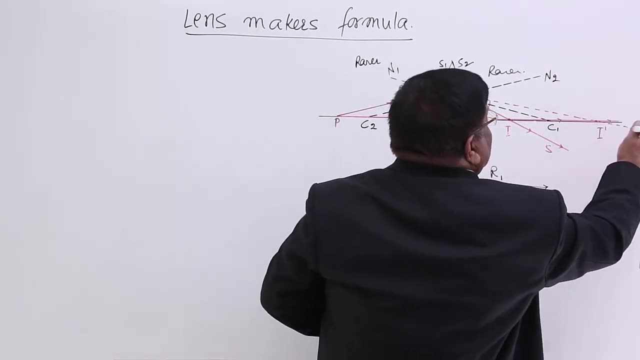 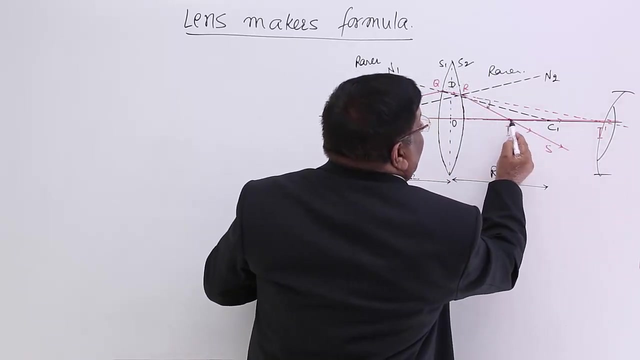 this path, it goes in this direction And on the way it intersects with this ray. Now, if we see this, put our eyes here. if we put our eyes here, where do we see? Answer is: one ray is coming from this direction. 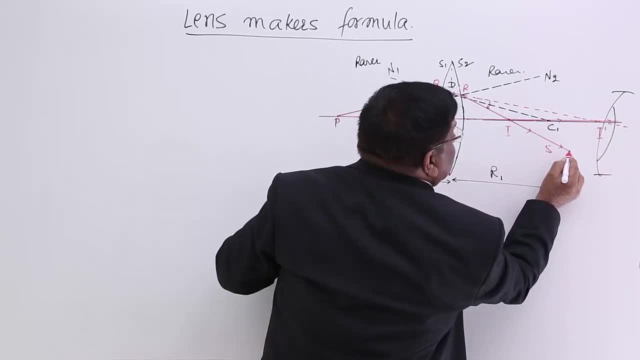 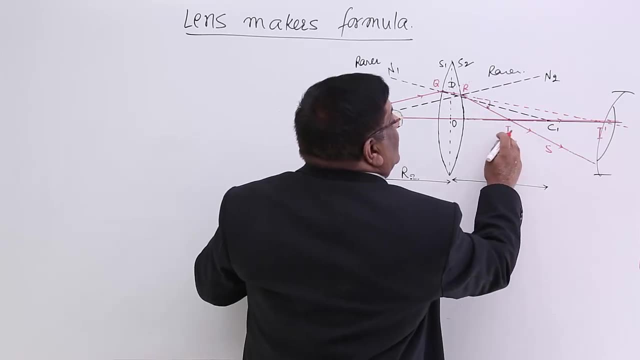 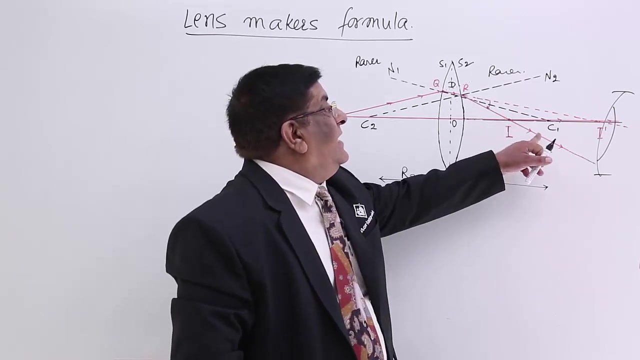 other is coming from this direction, and both the rays appear to come from a single point. And what is that single point? That single point is this: So we see image here, And this is a real image because they are actually coming from this point. 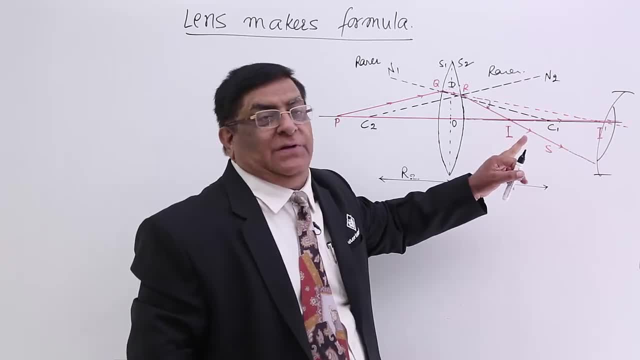 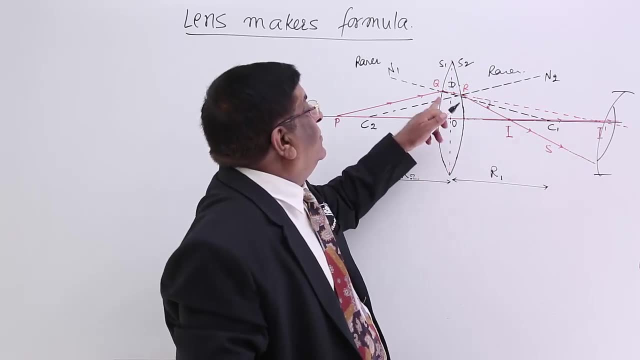 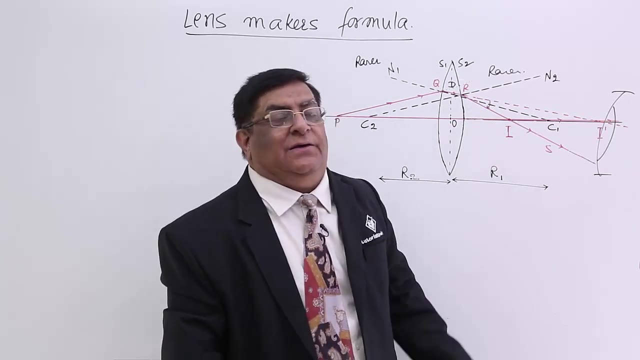 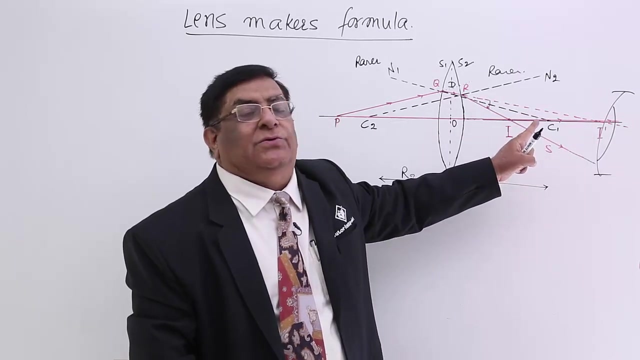 So this is finally when the image is formed. S1 tries to make it on I dash but because of this surface two, this has been sent to I. So we can say: S1 made an image at I dash and the surface number two for that I dash he replaced or he displaced that I dash to. 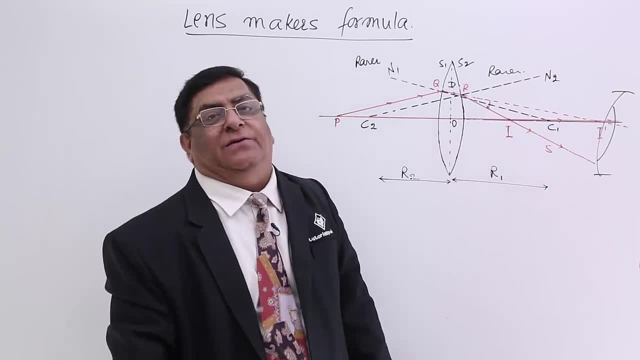 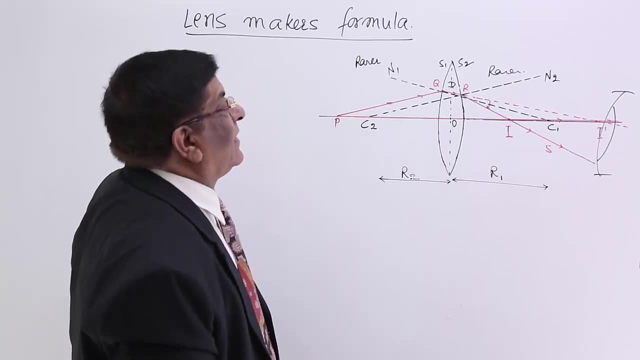 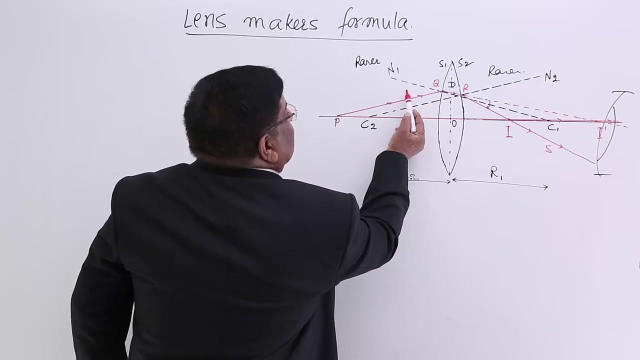 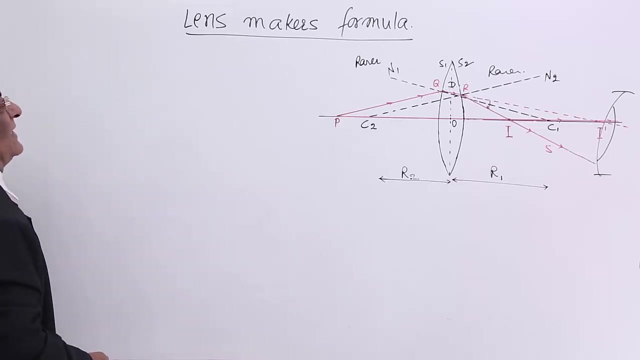 the point I and finally, the image was made here. This is what happens in a convex lens. Now coming to the calculations. First, this refraction has taken place. This is rarer to denser. What is the formula for rare to denser? 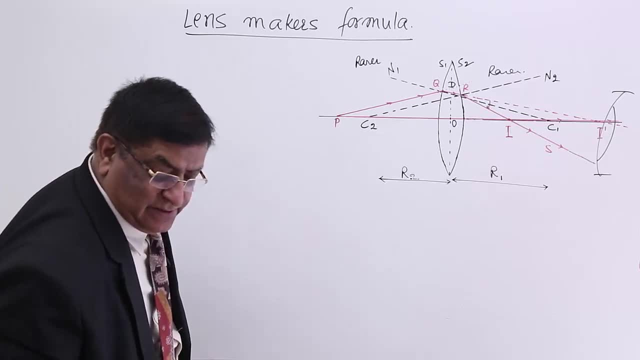 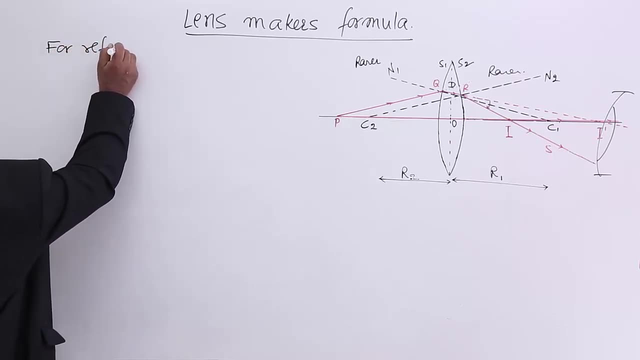 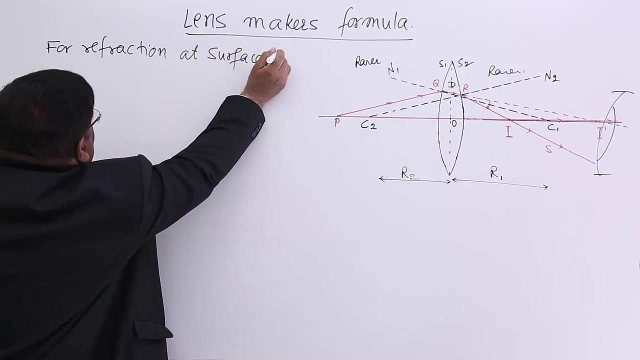 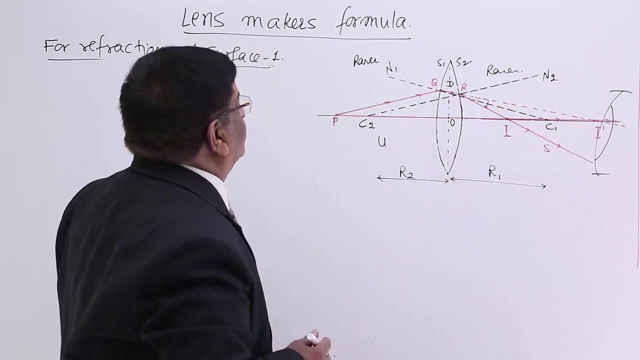 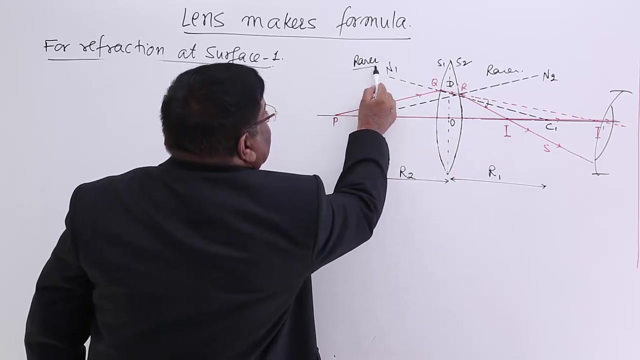 So for diffraction at surface number 1, for diffraction at surface 1, we know the formula. Now we do the calculation for this. There is a surface 1, this is object. the object is on the rarer side and on this side 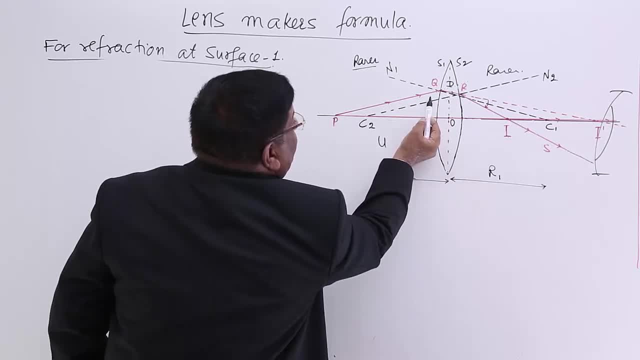 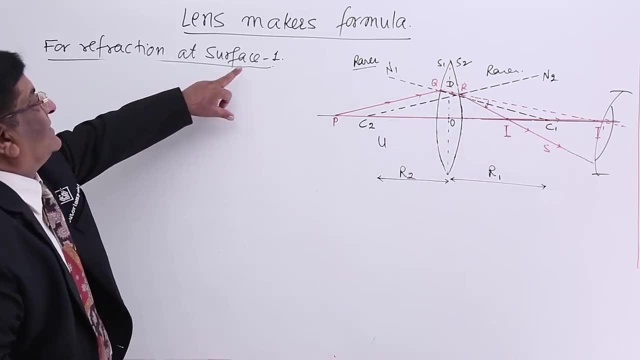 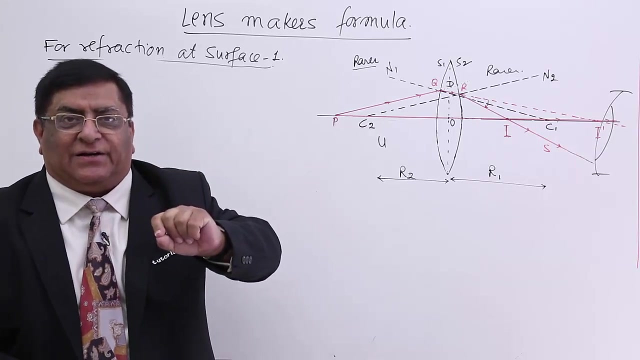 this is a denser medium, So there is a diffraction from rarer to denser and this is a spherical surface. So for diffraction at surface 1, what will be the rules applied? Spherical surface object is placed in the rarer. 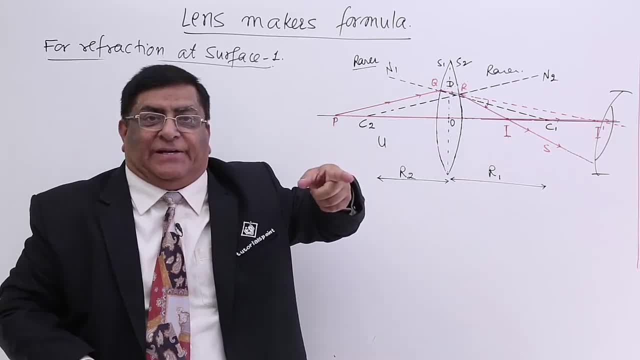 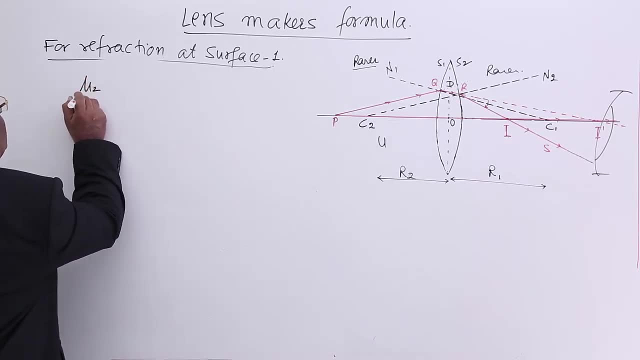 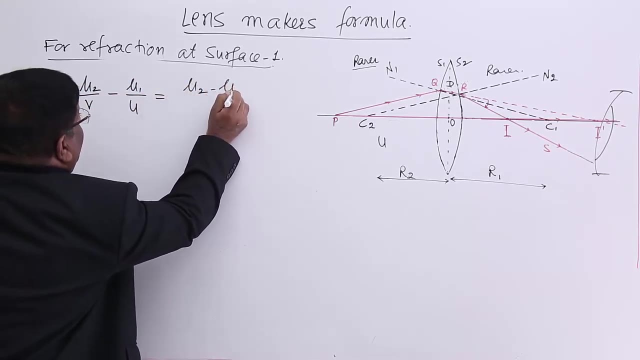 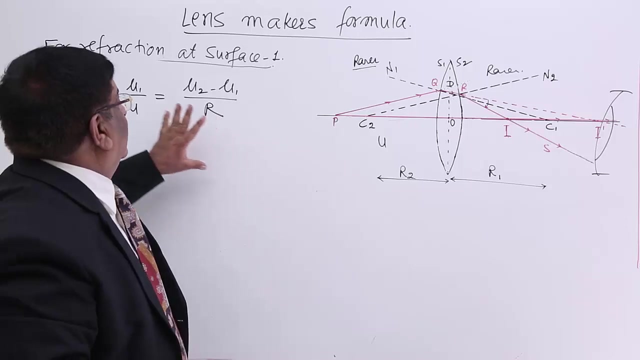 And image will be formed here in the denser medium. So rarer to denser, and what was our formula for that? That was: mu2 upon v minus mu1 upon u is equal to mu2 minus mu1 upon r. This was the relation for rarer to denser. 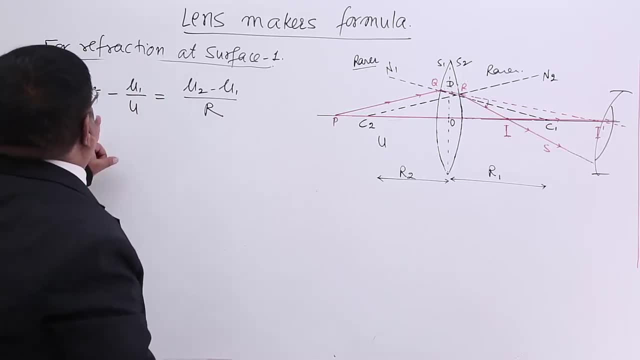 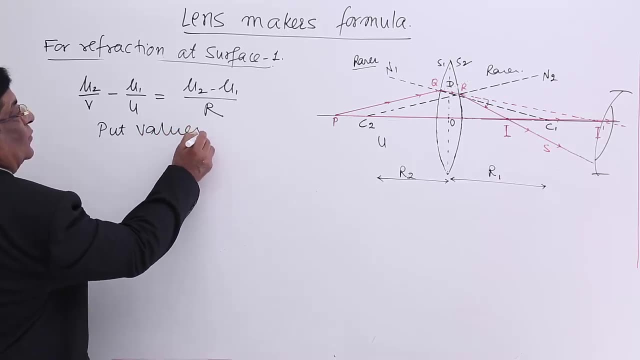 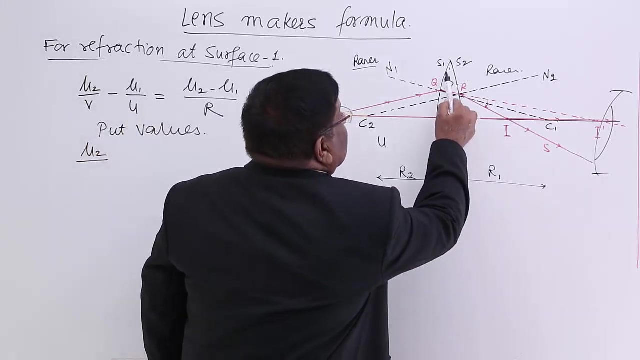 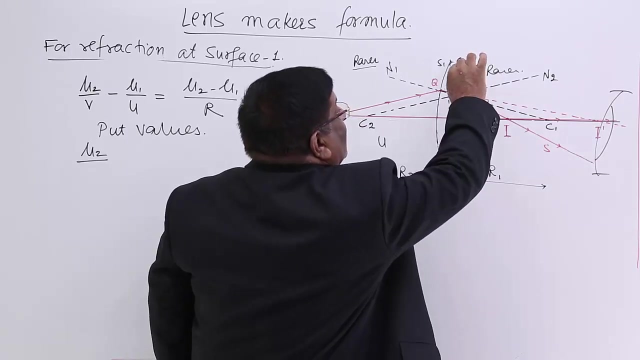 This we have done in the previous lecture. Now in this We put the values, put values here, mu2 upon v. What is v? This surface has sent this ray, this qr, and if there would not have been the surface, S2,. 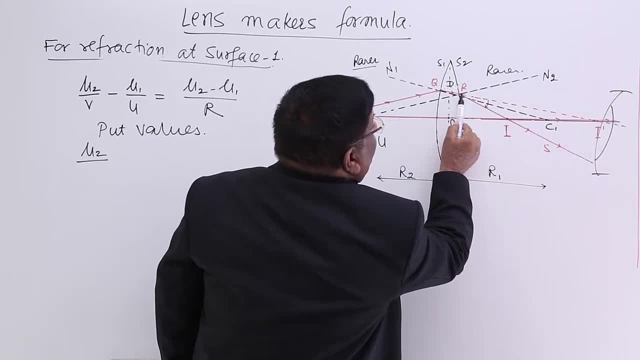 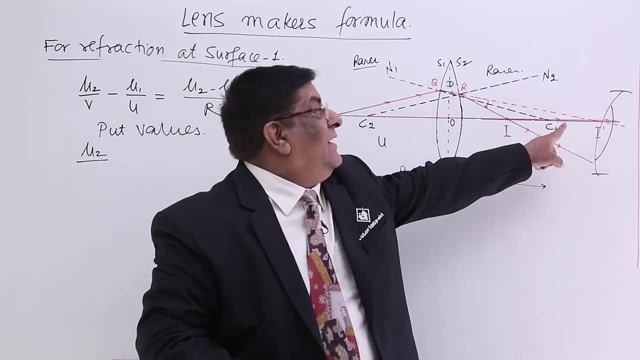 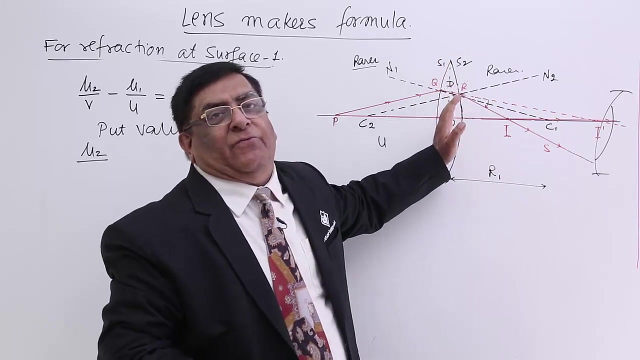 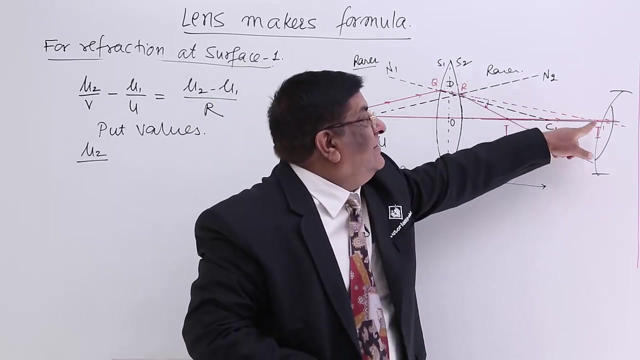 if this had been a full medium, then this ray would have gone to this point i dash And intersect with this ray where at i dash. So this was the direction decided by surface number 1.. So, as far as surface number 1 is concerned, it has sent the ray to make image at i dash. 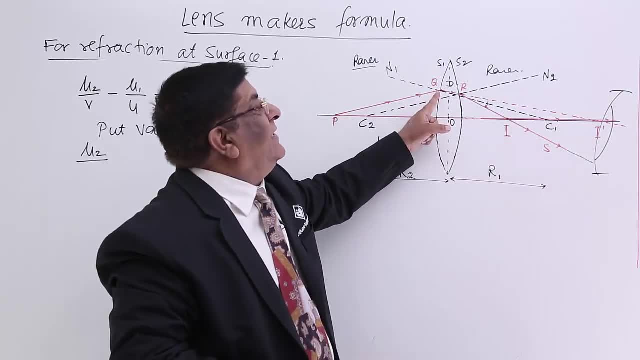 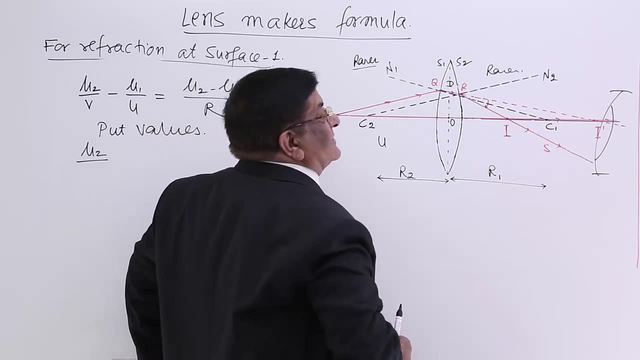 So for this surface, number 1 diffraction image is to be taken at i dash. So what will be the value of rarer to denser? So rarer to denser Distance of image o to i dash, and this is on the right side. 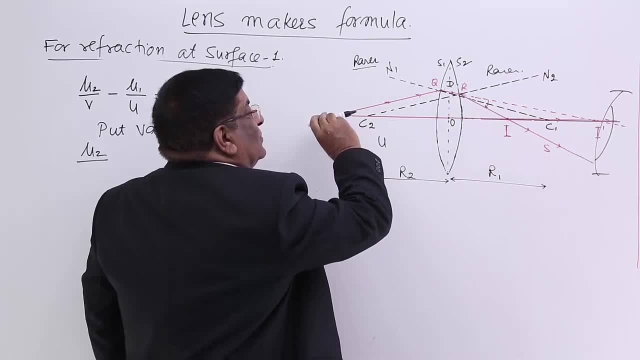 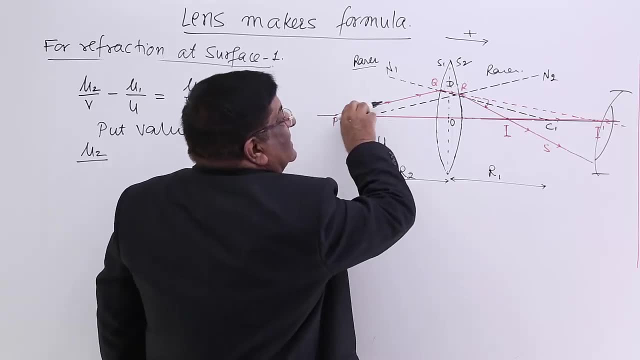 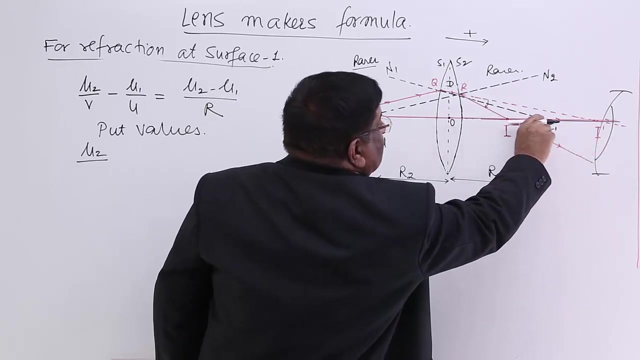 This is on the opposite side of incident ray. sorry, This is direction of incident ray. So this is the direction of positive, the direction of incident ray. So from origin o on the right hand side, this is positive distance o to i dash. 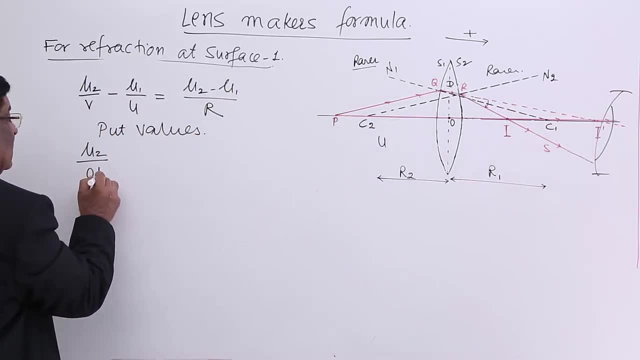 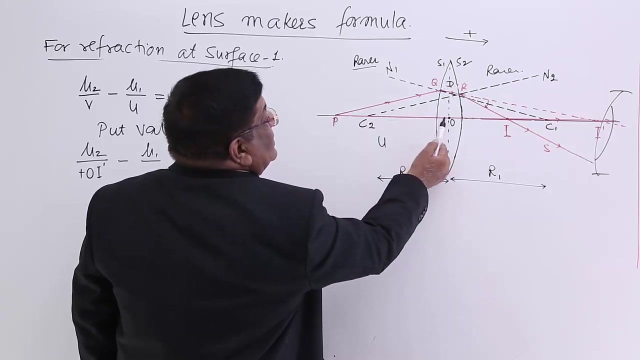 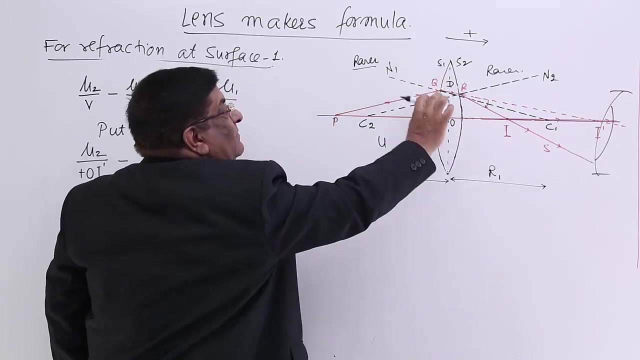 So we write it o, i dash, and this is plus minus mu 1, u. u is the distance of object for surface, number 1.. This is u, or we can take it from here: o to p, and this is on opposite side of the positive. 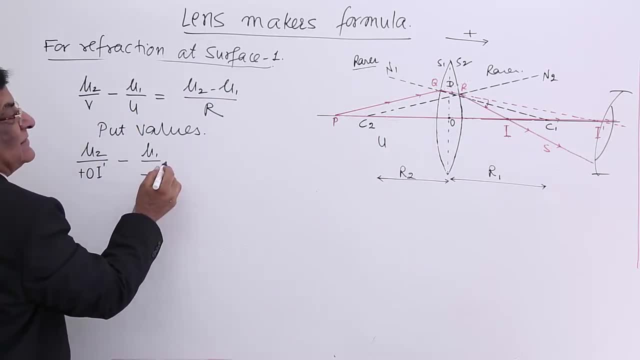 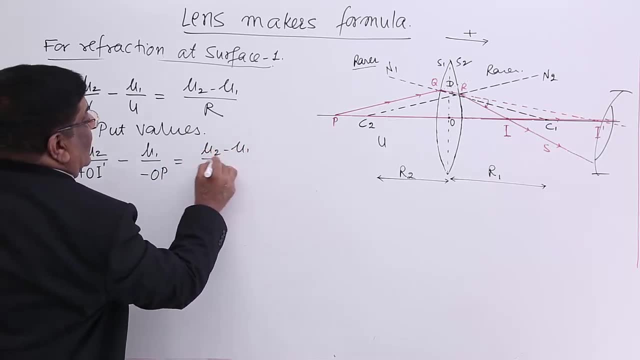 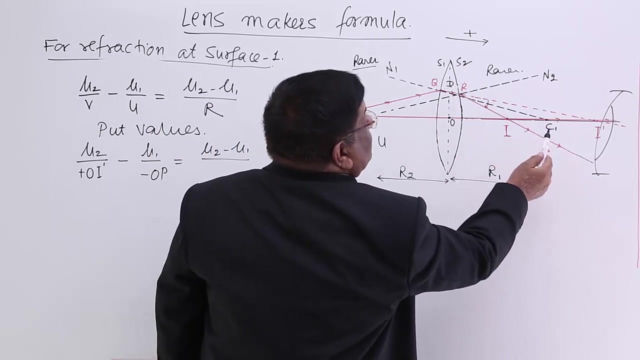 So this is minus, This is minus o p o p o p? u is equal to mu 2 minus mu 1.. Radius: What is radius of the surface number 1?? Radius of the surface number 1 is c1 is the center. 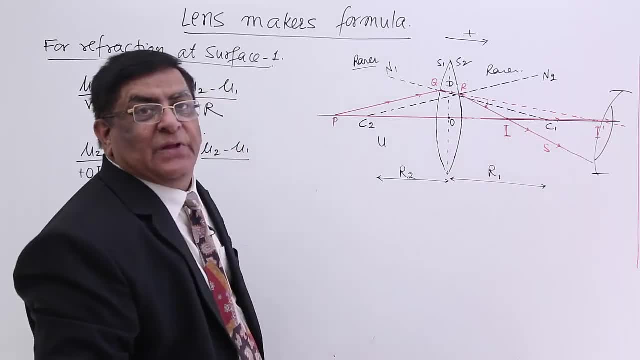 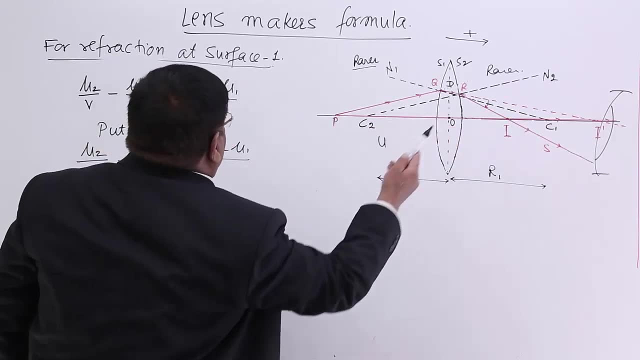 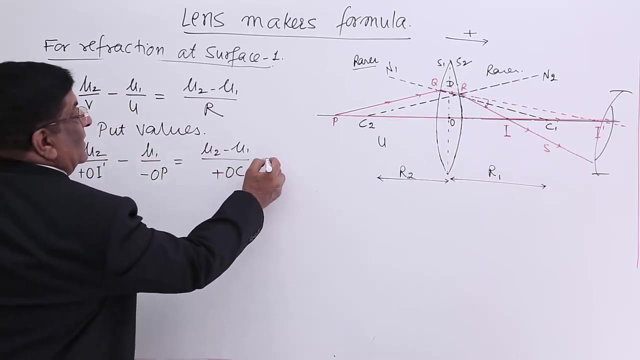 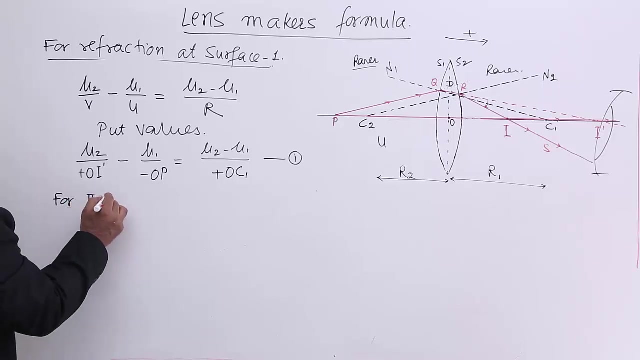 So o to c1 is the radius. So we will write here: o to c1 and what is the sign it is carrying? It is carrying positive sign. So this is plus o c1.. This is equation 1, we stop here. now we go for second refraction. for second refraction. 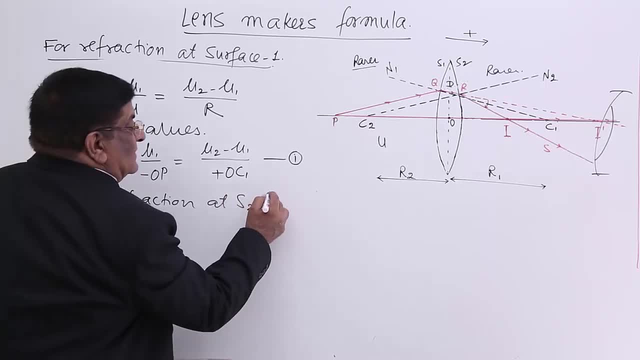 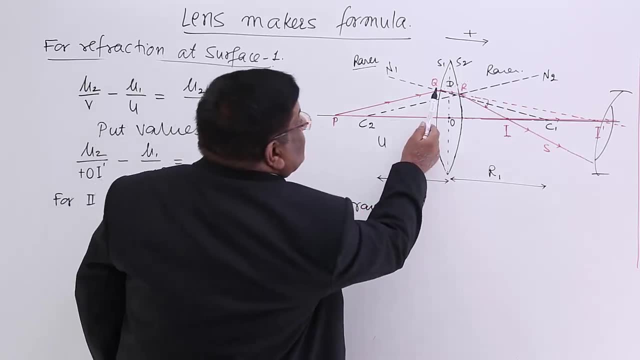 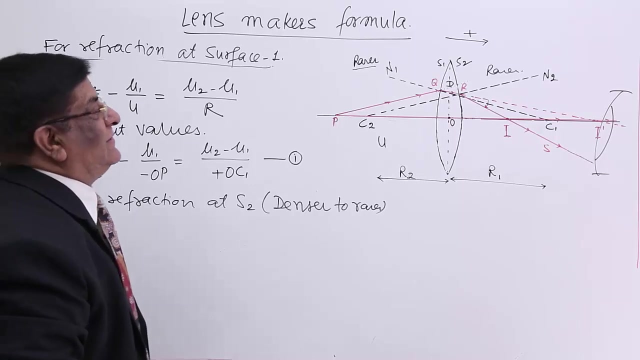 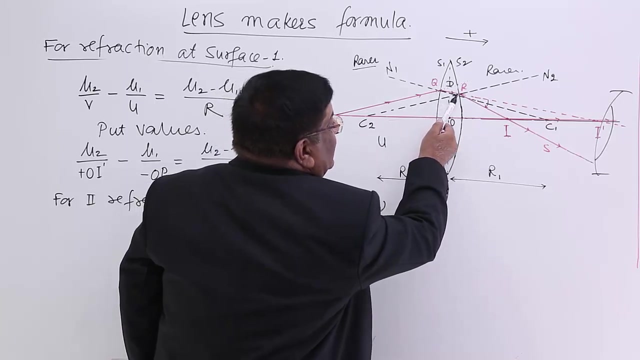 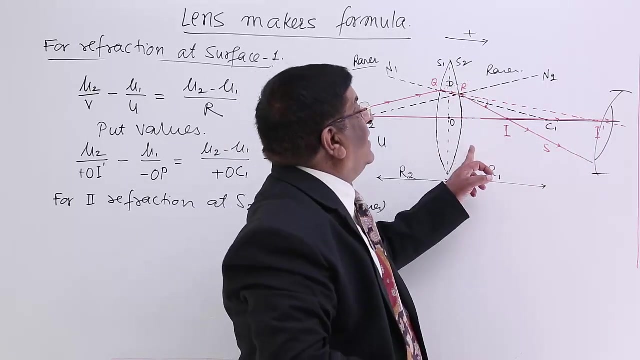 at surface 2, and this is what denser to rarer, because this is denser, this is rarer. So denser to rarer. and what is the object? what is the surface S2 is doing? S1 has sent the light ray to form an image at I dash, when there is a surface 2, surface 2 has displaced. 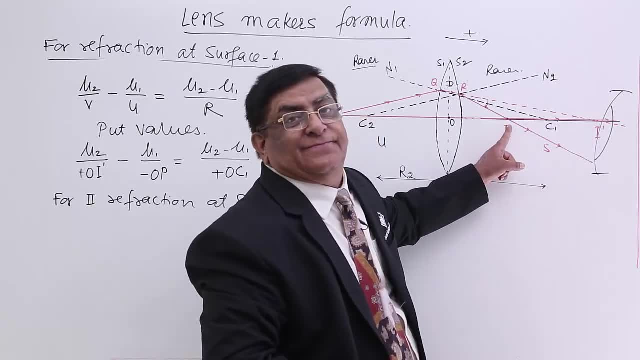 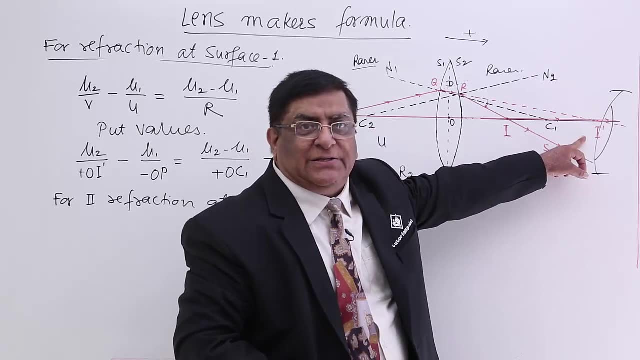 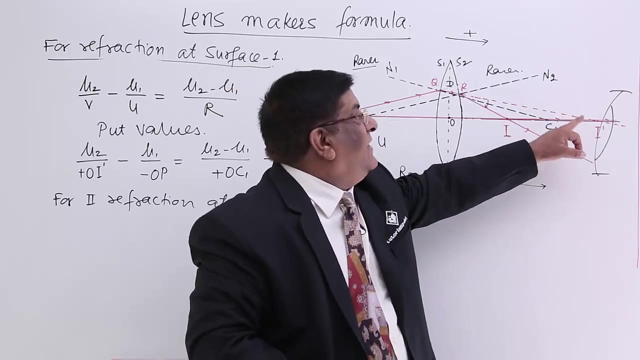 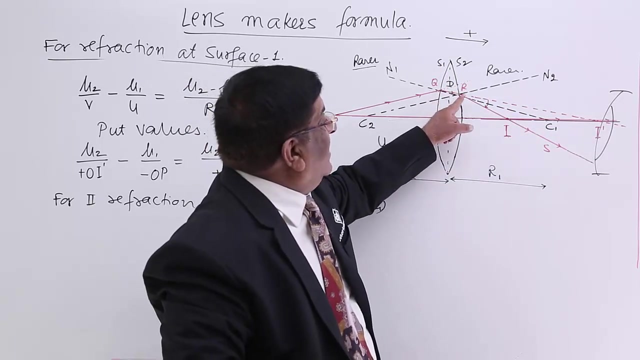 I dash to make the image at I So for surface number 2, we will assume that I dash was the object Which he has pulled to I. So this is object for surface number 2 equation and this is image. again, this is the incoming. 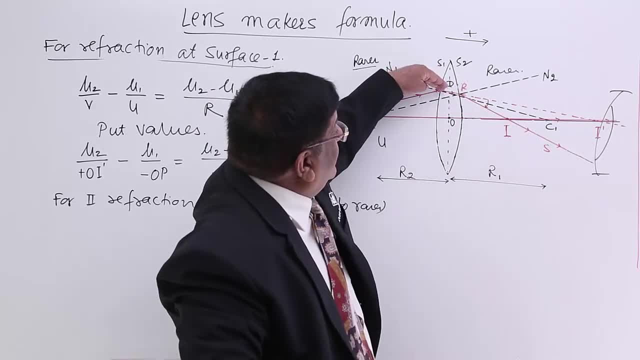 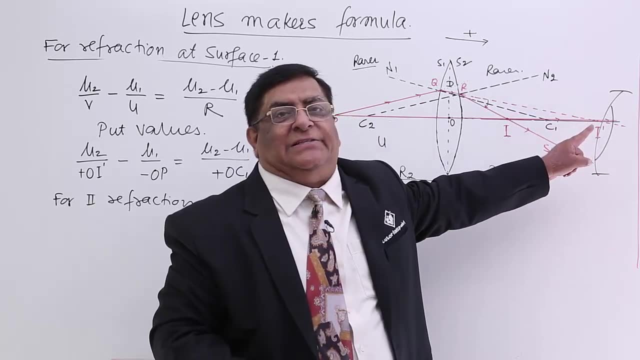 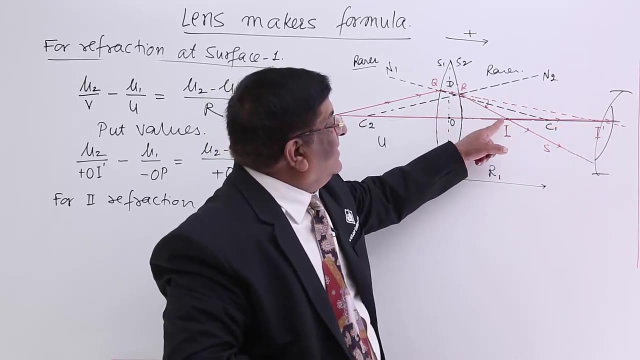 ray. this is refracted ray, so incoming ray intersect with the principal axis at I dash. therefore I dash can be taken as a position of object. incoming ray intersected object Outgoing. the refracted ray intersect at the position of image. so this is image. this 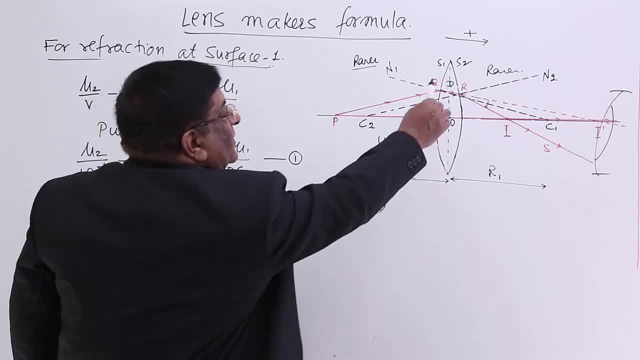 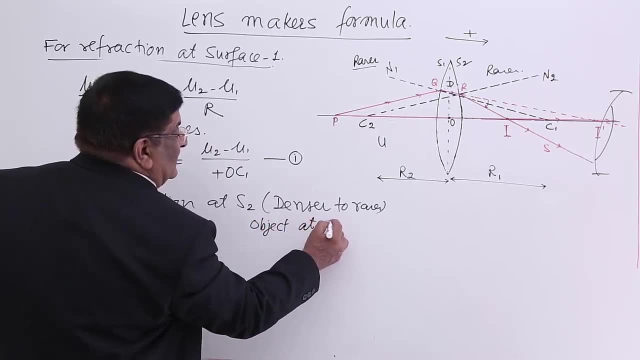 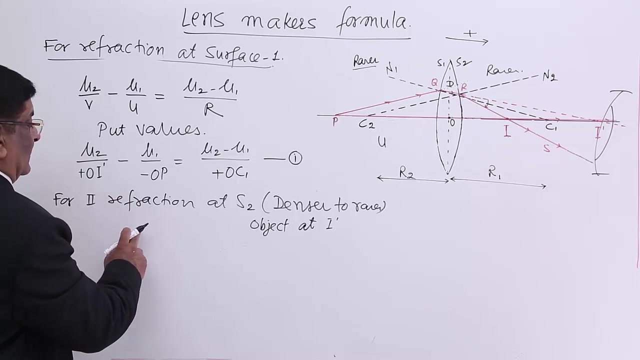 is object. Now, this is for the second. so object at: I dash. Now. what is the relation for denser to rarer? so, denser to rarer, we relation. right, that is mu1 upon v. here it is changed in place of mu2. it is mu1 minus mu2 upon u, mu1 and. 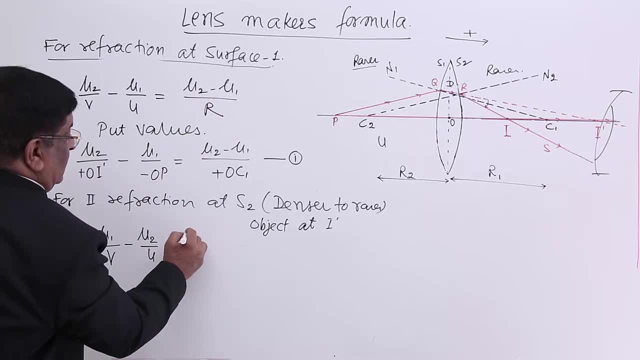 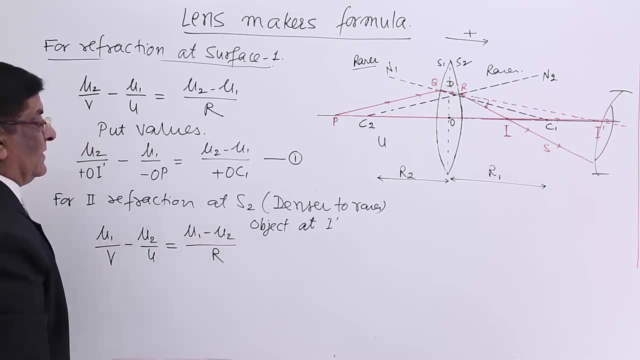 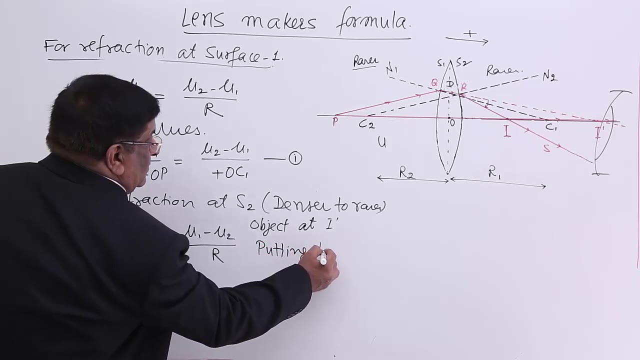 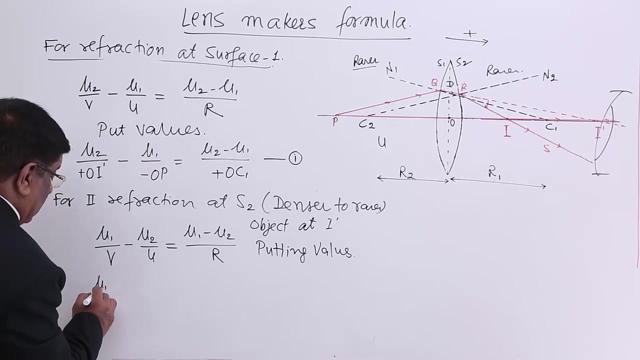 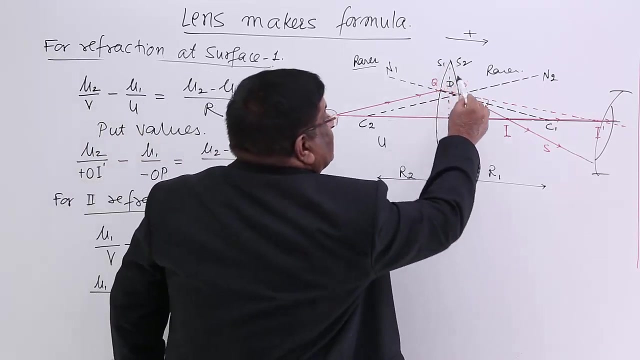 mu2 are exchanged, this is equal to mu1 minus mu2 upon r. this Now put values. Ok, Putting values. now we put geometrical values: mu1 upon v, v for dot v, for second refraction, For this refraction. this was the object, this is the image. so what is v? o into? i? 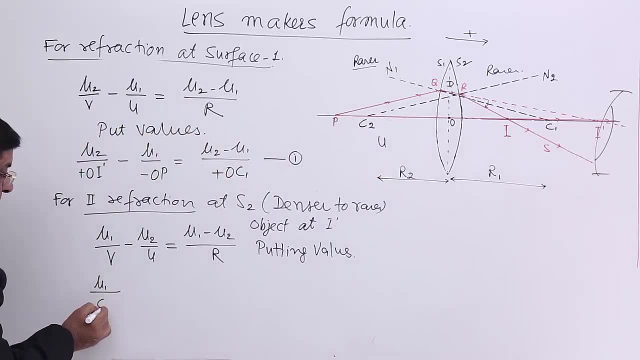 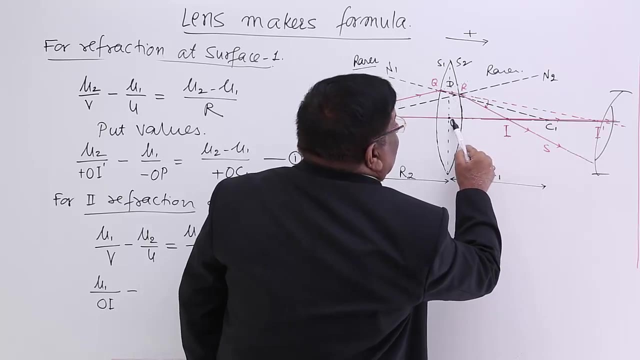 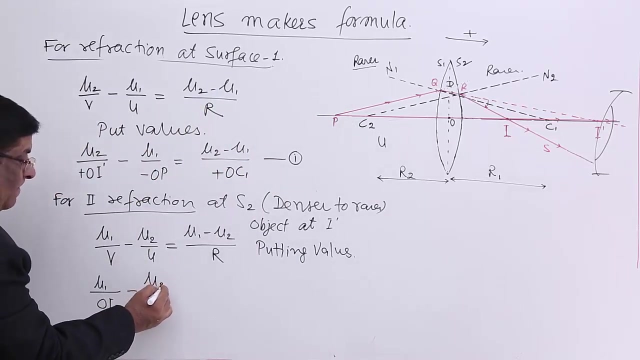 on the right side. So this we can write as: o i Ok, Then minus mu2 upon u. this was the object for this second refraction and this is o i dash, but it is again on the positive side. So this is mu2 upon o i dash. this is equal to mu1 minus mu2, mu1 minus mu2 divided by: 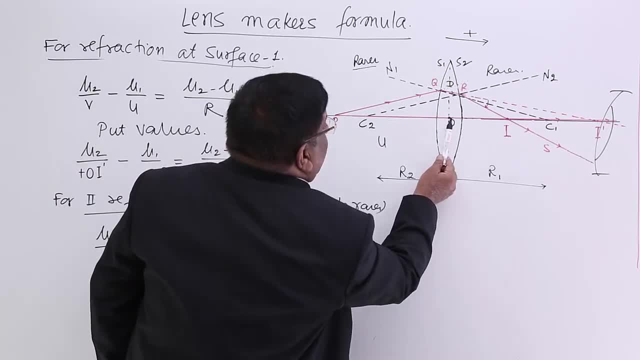 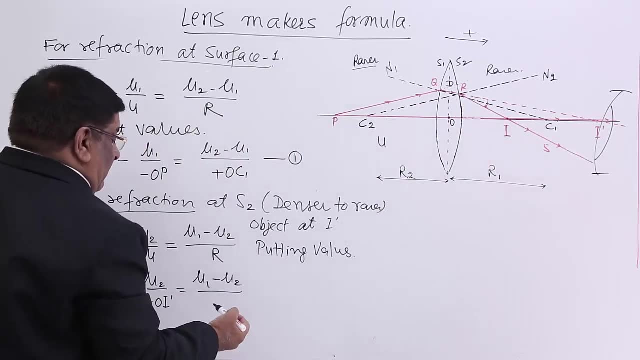 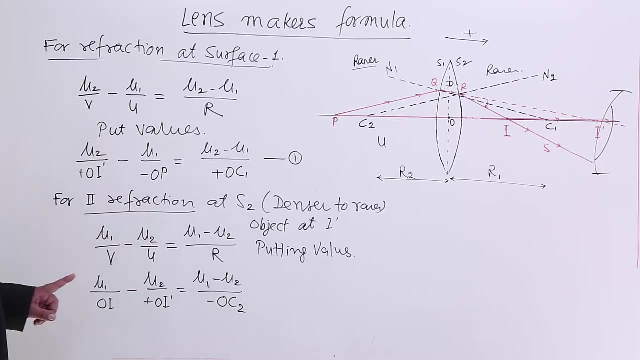 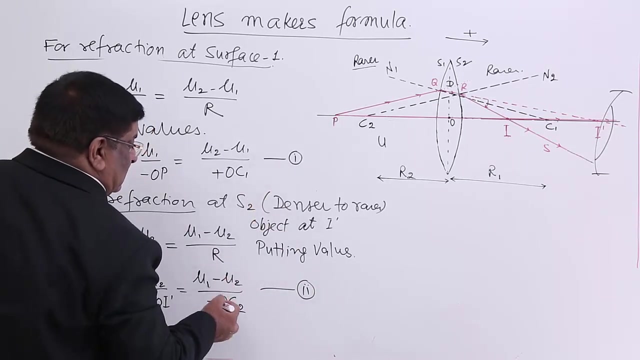 radius. radius of surface. number 2 is oc2.. But this is on left side and here is the positive direction. it is in this direction, so this will be minus oc2.. Ok, Now, these are the two equations. this is for refraction 1, this is for refraction 2.. 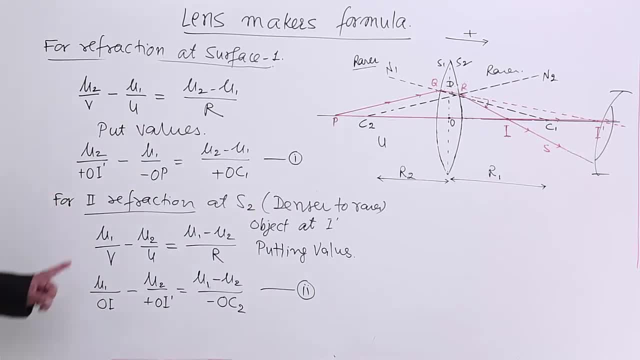 Now We do certain operations in this. this we simplify minus into minus. this will be plus, so we write it plus and omit it. okay, Now this is already plus, we need not write it. this is minus into plus is minus, okay. 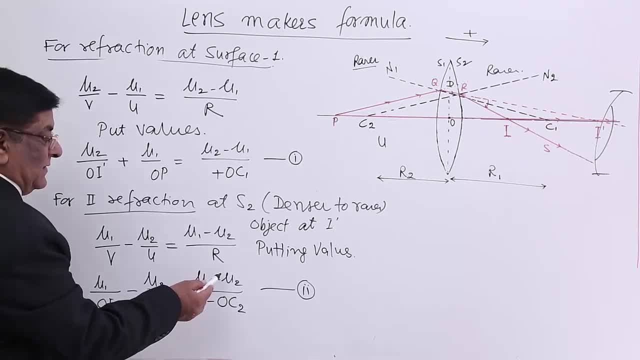 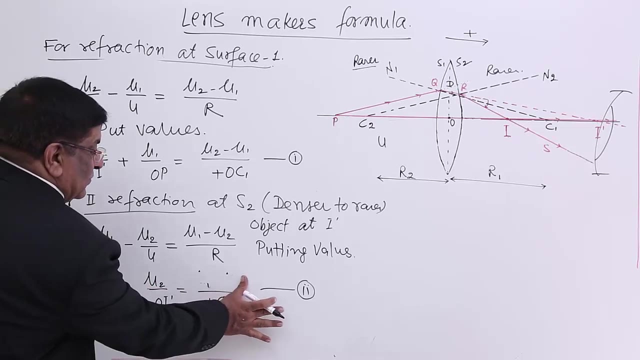 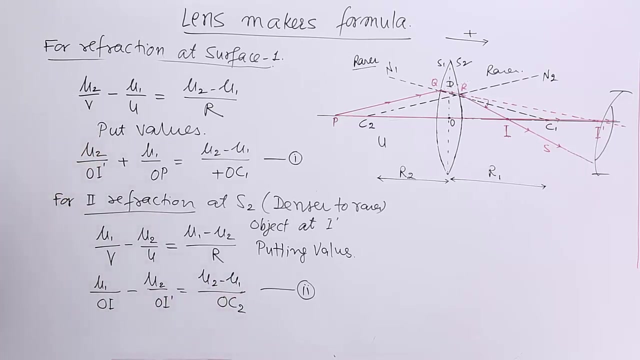 Now this is minus. if we multiply minus here and here both sides, so this will be plus, minus and this will be plus. we can write it this way. So then this will be mu2-mu1, so I write it: mu2-mu1 upon oc2,. this is simplified. 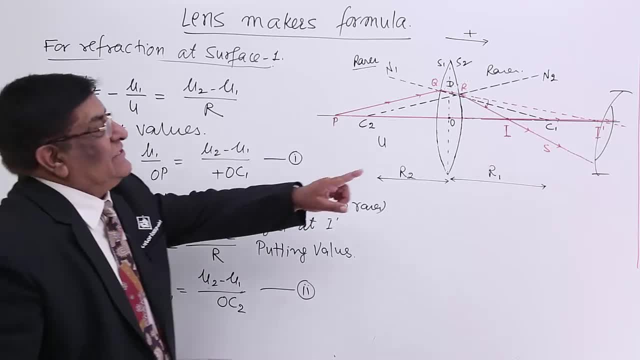 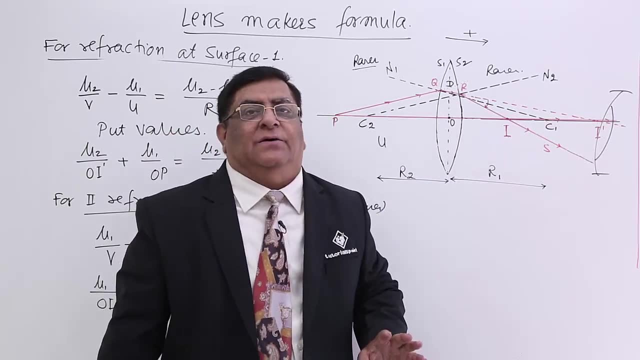 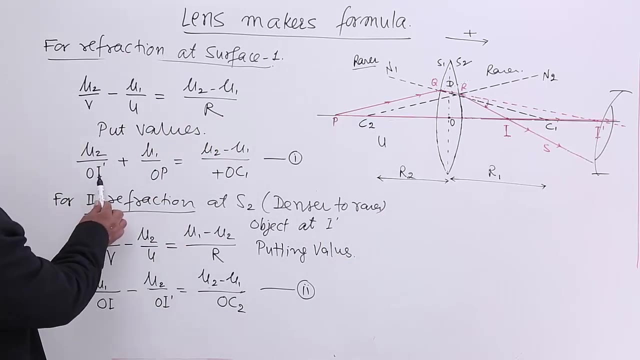 Now we add the 2, why i dash is imaginary. we want to clear out, we want to delete the terms which has got i dash Here. this is i dash here. this is i dash: mu2 upon oi dash plus. mu2 upon oi dash minus. 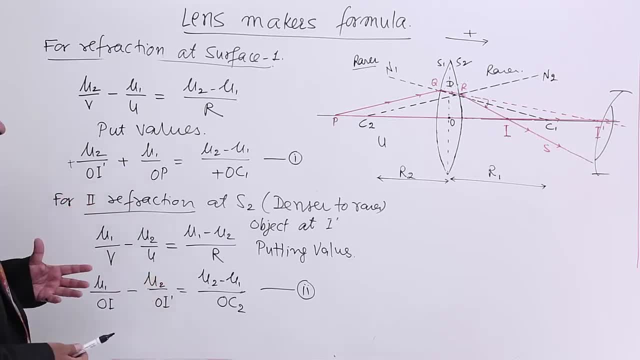 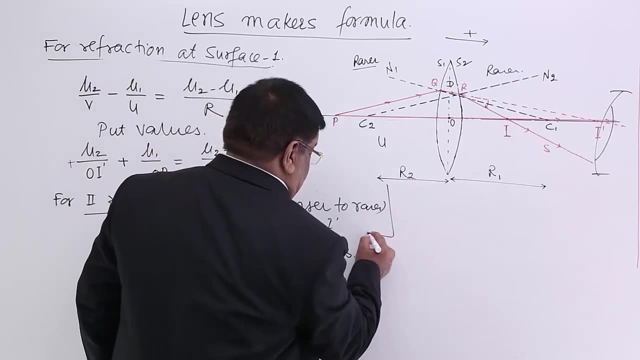 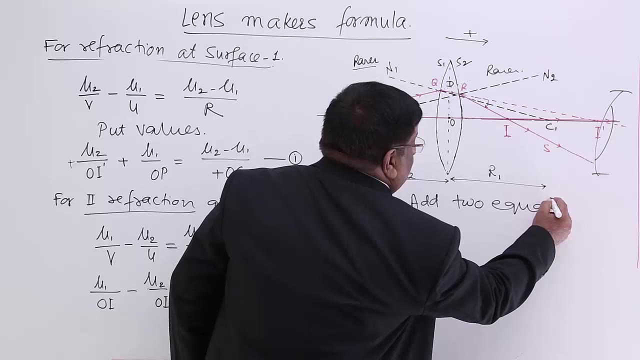 if we add these 2 equation, this will be omitted, and that is always remember. we have to do it this way. So we add the 2 equations, add 2 equations. Now we add 2 equations, and what do we get? 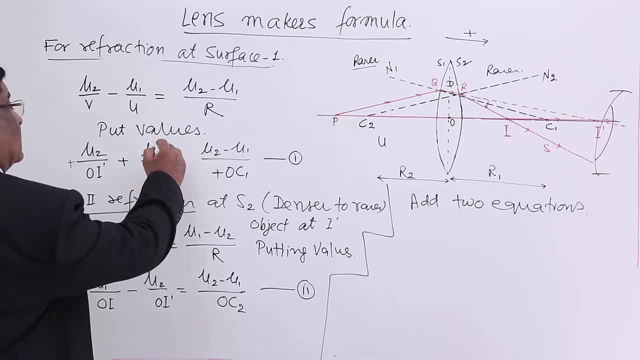 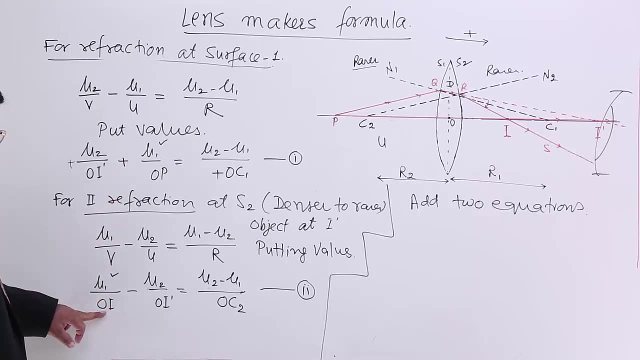 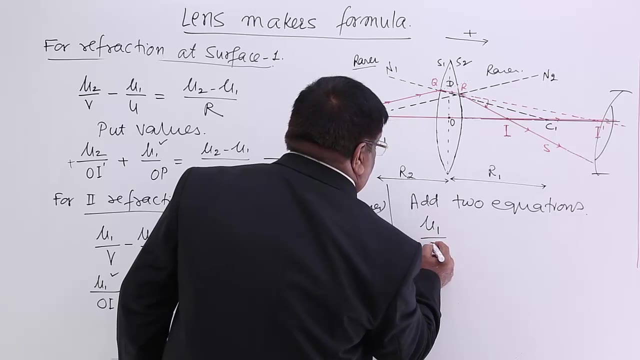 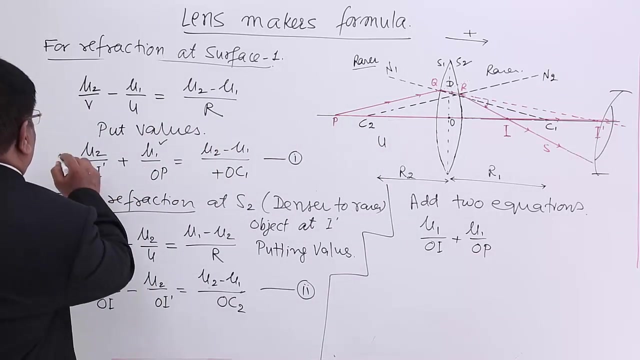 These 2 are getting cancelled and these 2 are remaining, so we write them: mu dash upon oi, This is mu1.. This is mu1 upon oi plus mu1 upon op plus mu1 upon op. done. done. These 2 are cancelled is equal to add the 2.. 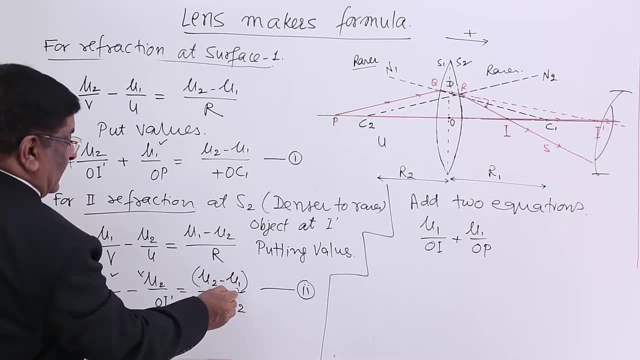 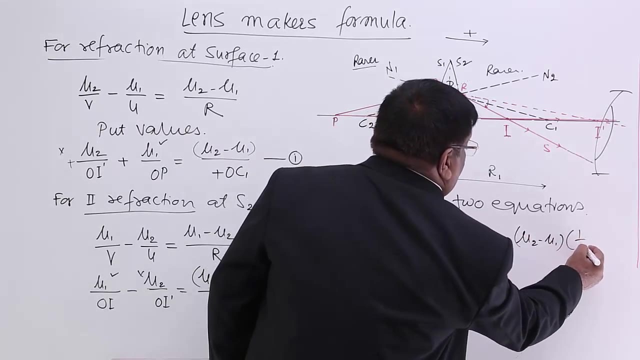 When we are going to add the 2, we are getting a common term, mu2-mu1 here, and here we take it out. So this will be 1 upon oc1 upon. so this is mu2-mu1, 1 upon oc1 plus 1 upon oc2, yes, 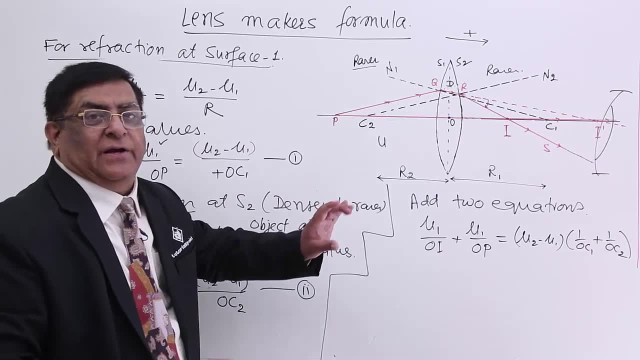 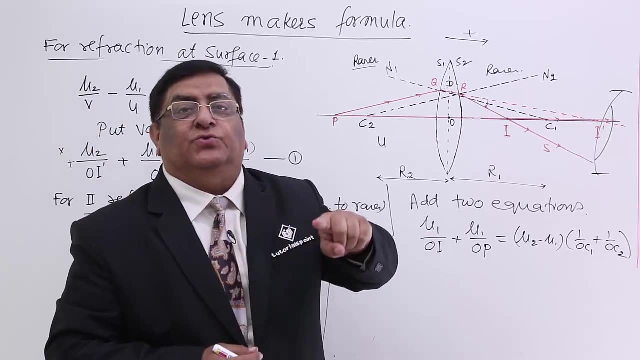 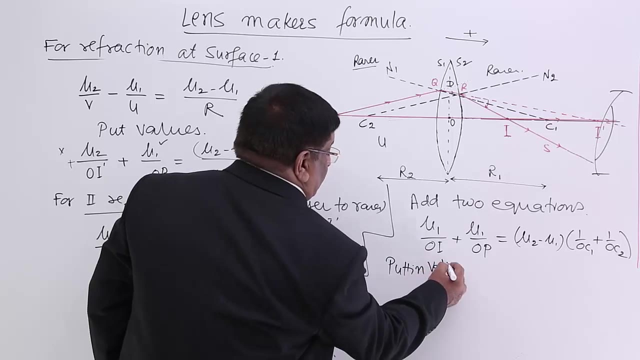 Okay, This is the geometrical equation we got. Now we again convert it into optical terms, Optical terms which are having u, v and r. Okay, Okay, So this is. we are putting values. What values? oi, oi is what? 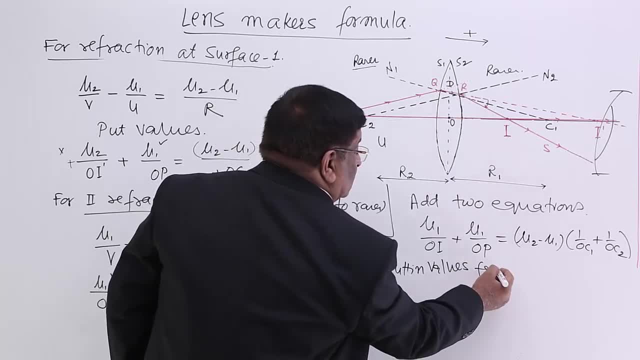 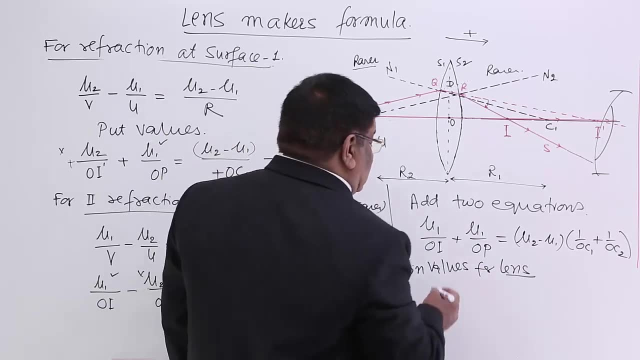 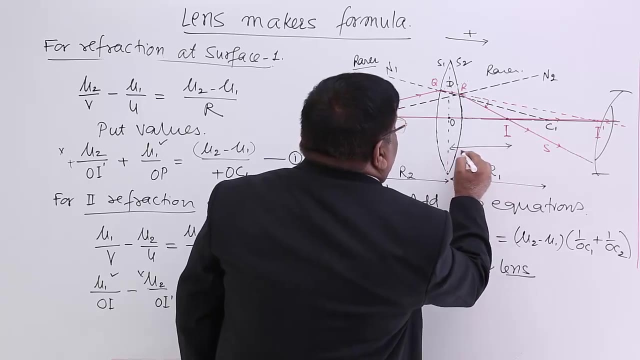 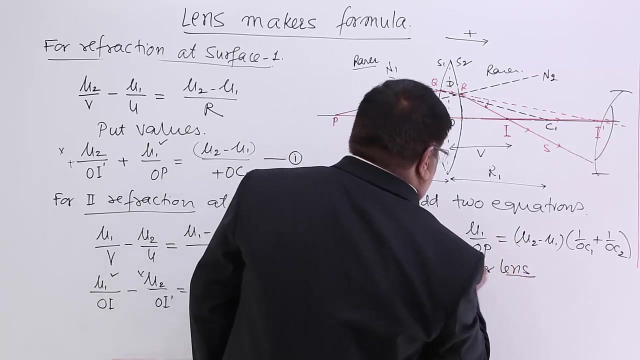 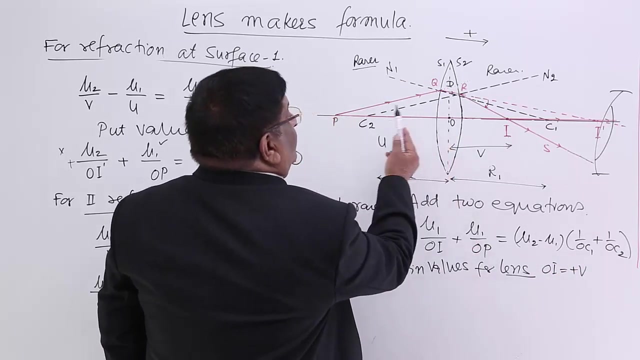 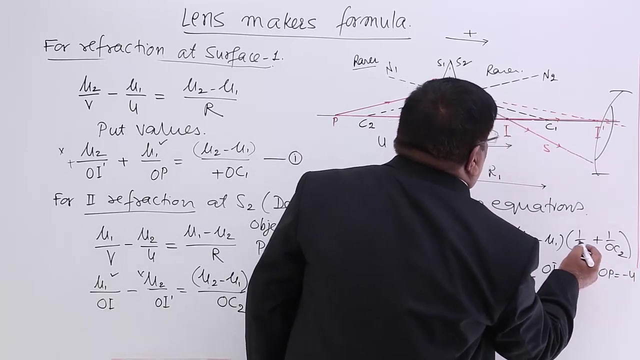 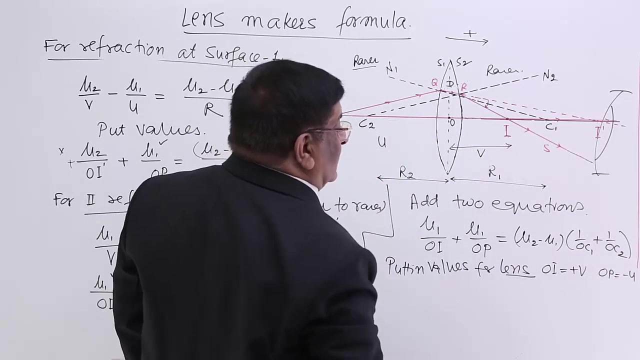 For this lens, Putting values for lens. Now, it is not for the surface, It is for the lens. So for lens, oi is equal to final image at a distance, v. So This is for the lengths. oi is equal to plus v, op is minus u, oc1 is plus r, oc2 is minus r2.. 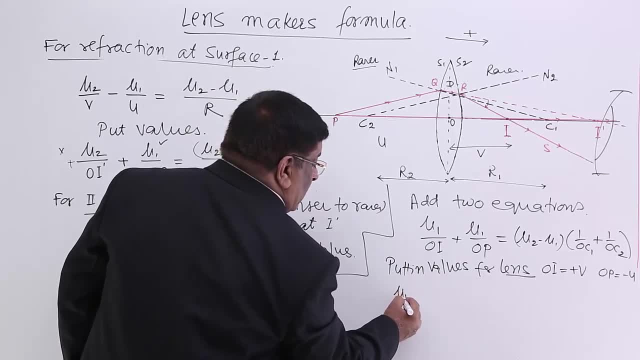 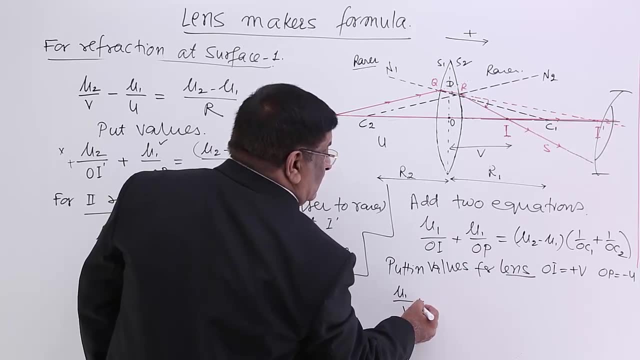 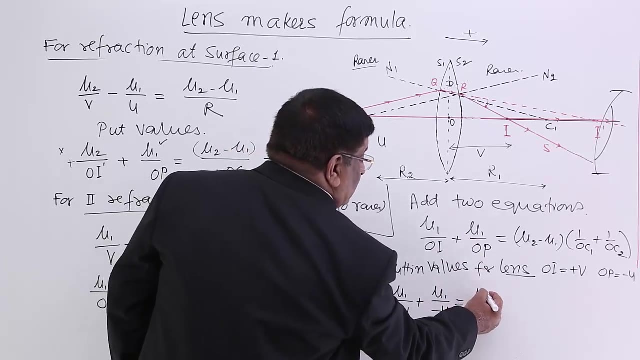 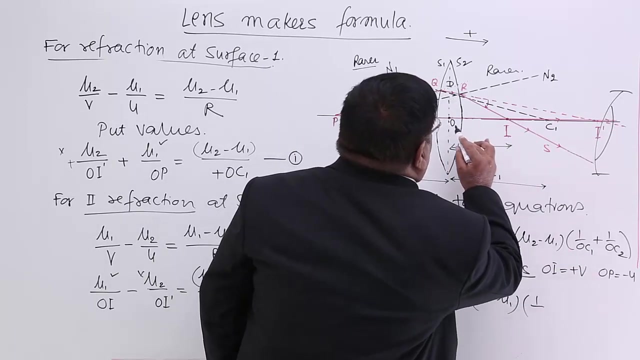 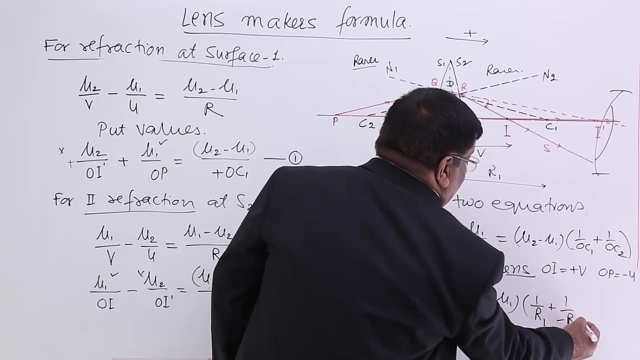 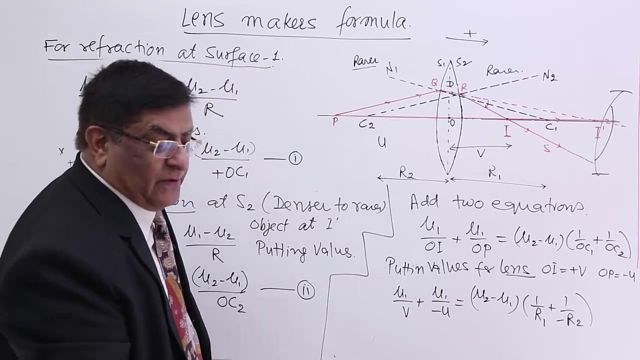 So now this will become mu1 upon v. This is plus mu1 upon minus. u is equal to mu2 minus mu1, multiplied by 1 upon oc1 r1, and this is 1. upon minus R2, okay, Again, we write it clearly and simplify this. When we simplify this, what? 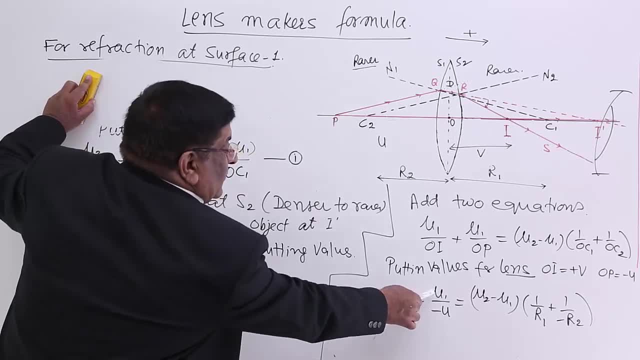 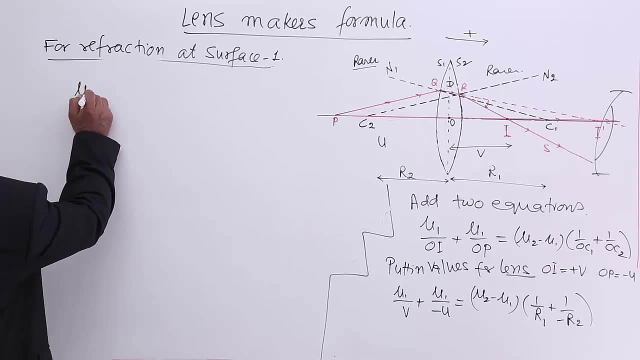 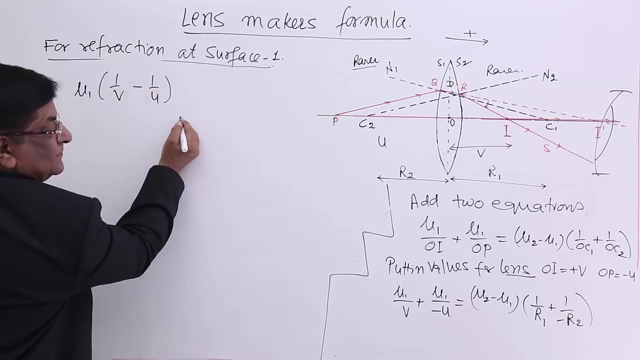 we see mu1 can be taken out from here. okay, Now this we will write here simplified: mu1 is taken out, So this is 1 upon v minus 1 upon u. This is equal to mu2 minus mu1, mu2. 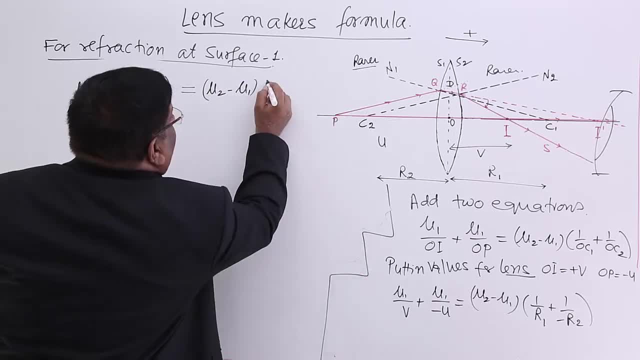 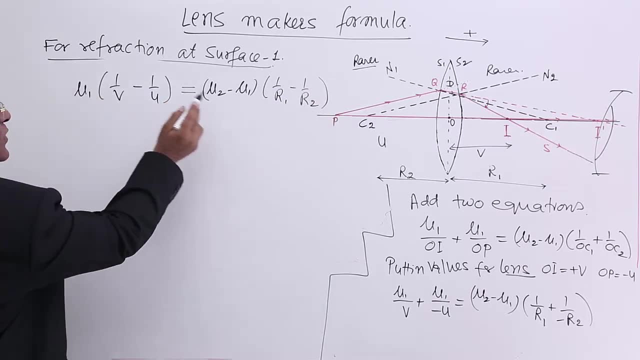 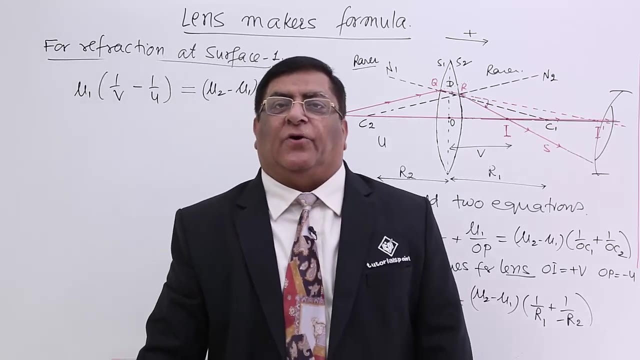 minus mu1, 1 upon R1 minus 1 upon R2.. Take this mu1 on this side, Now this 1 upon v minus 1 upon u for a lens, We can prove that for a lens, 1 upon v minus 1 upon u is equal to 1 upon f. That is its. 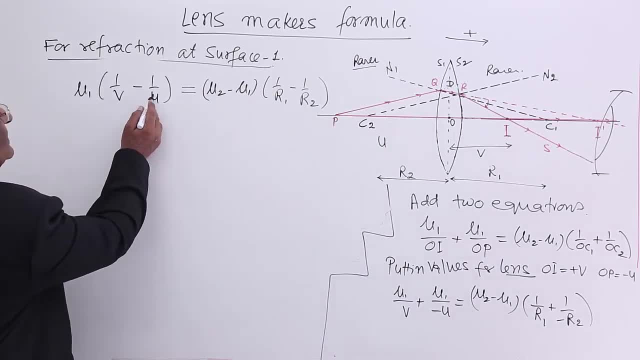 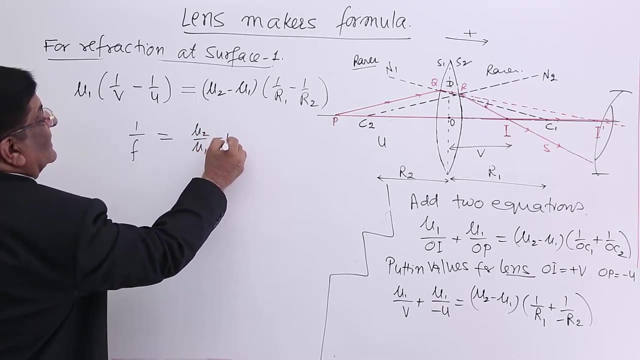 definition. So this 1 upon v minus 1 upon u is converted as 1 upon f. This is equal to mu1. has come here. We will divide it with mu1.. So what this will be: mu2 upon mu1 minus. 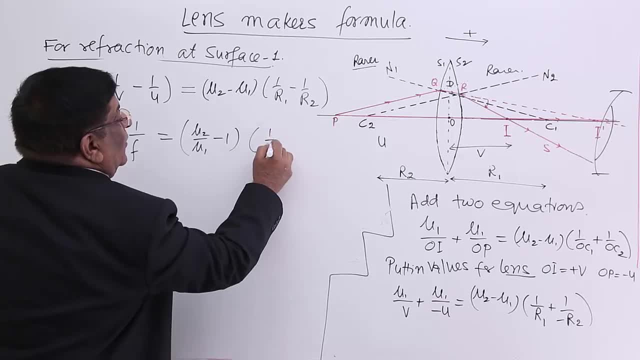 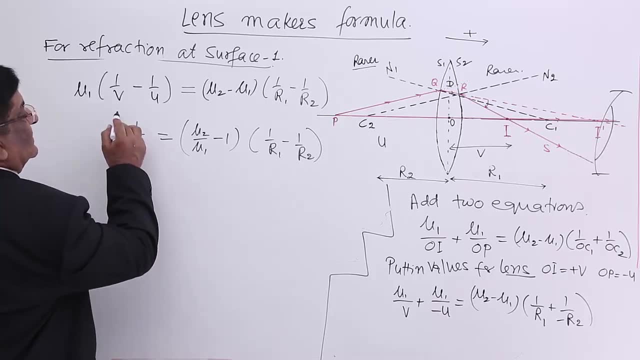 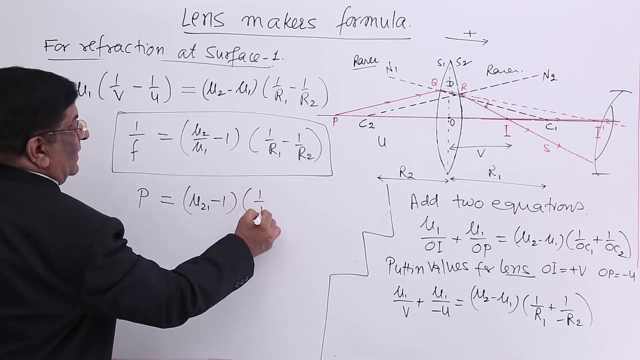 1.. This is 1 upon R1 minus mu2.. This is 1 upon R1 minus 1 upon R2.. So now our formula stands this one: If we say 1 upon f is equal to power, then this is power. mu2 upon mu1 can be written as mu2, 1 minus 1, 1. 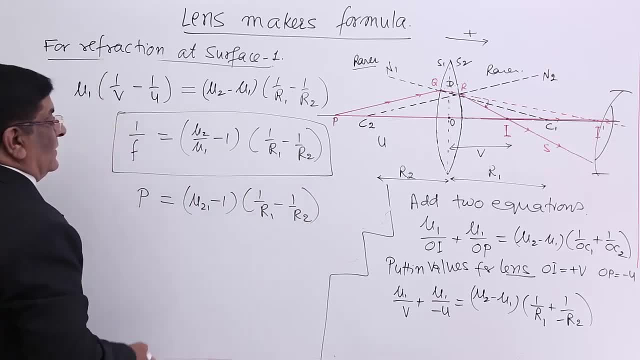 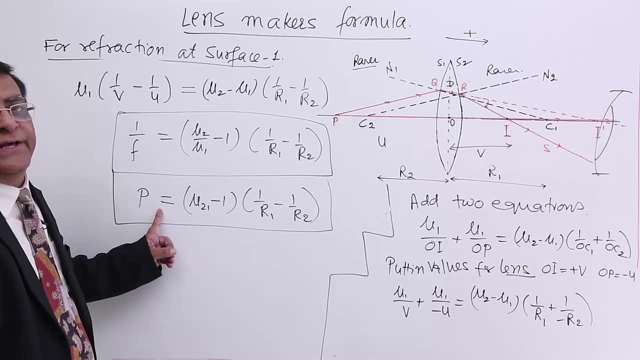 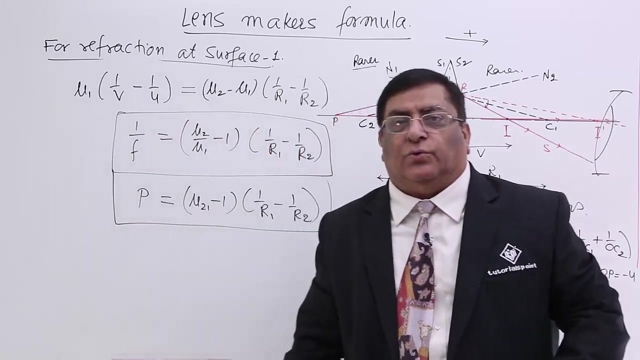 upon R1 minus 1 upon R2.. Now, which are the quantities involved? The power for which we give order to the lens maker, Mu, is that material which he is filling up in the lens, For that refractive index is mu. Radius one and radius 2 are the radius of 2 dice. So 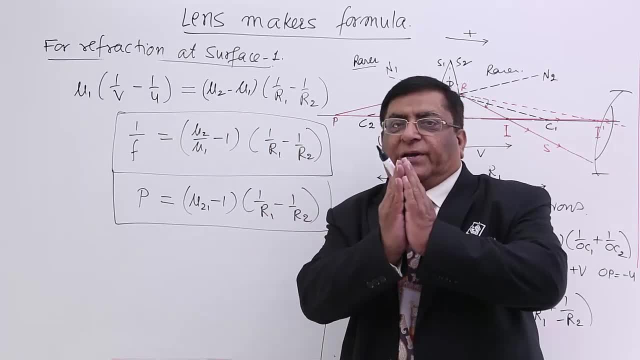 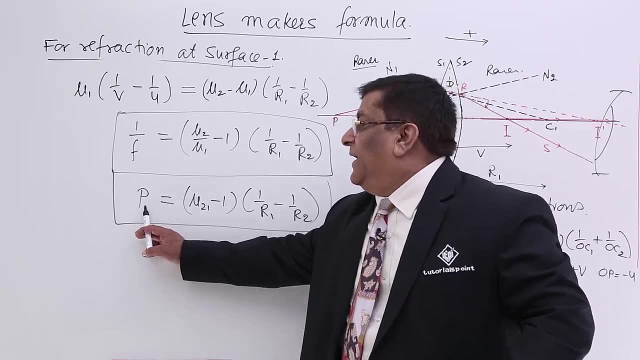 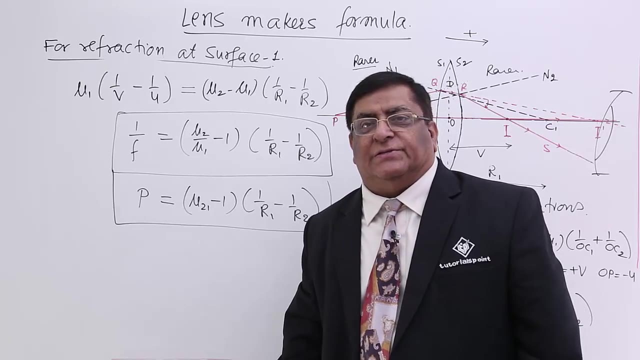 when we put the 2 dice together with radius 1 and radius 2, and fill up the material of this refractive index, you will get a lens And the power of the lens will be given by this relation. And whenever we solve numericals based on this, all this R1 and R2 has to be placed. 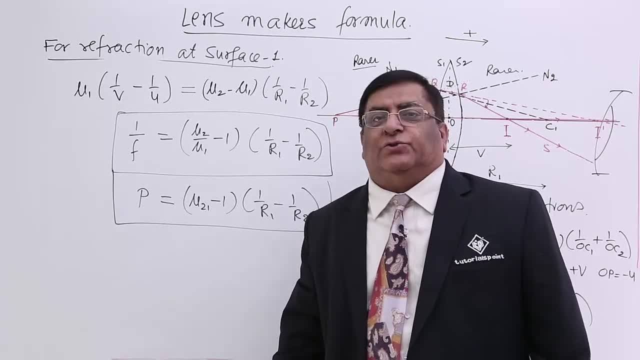 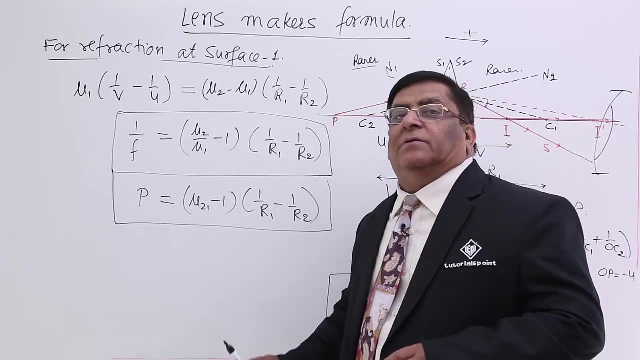 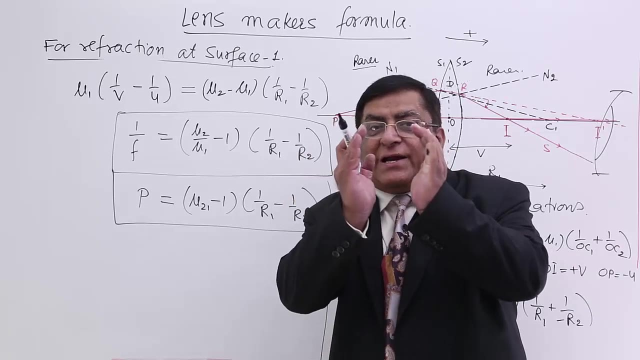 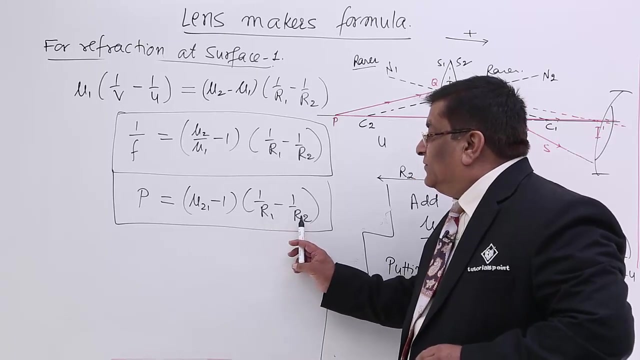 with sign that is required. So when we make the numericals of this, you will see that if R and R- both are equal- they will not cancel each other. Why? Because one R is always positive, one is negative. So if both R has got value 10 cm and 10 cm, for this you will place plus 10 and for this